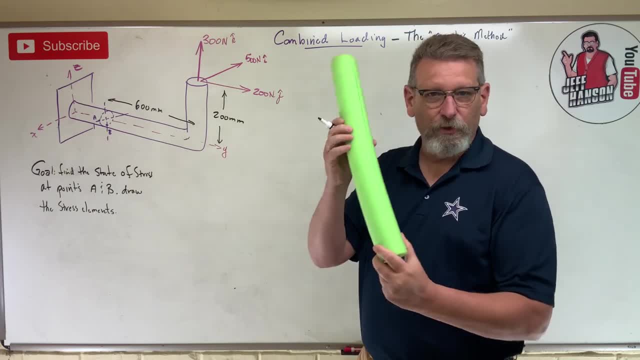 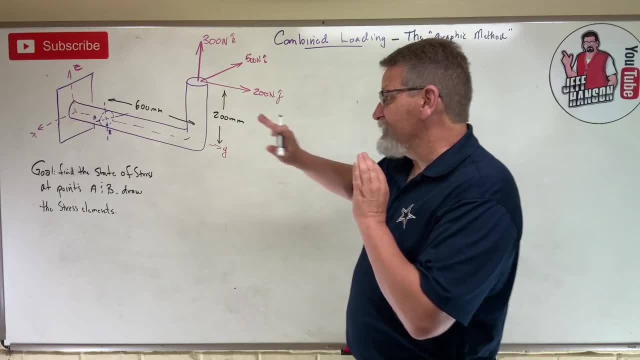 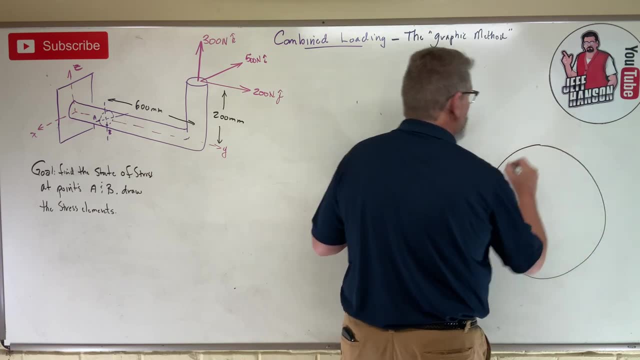 do. okay for the graphic method is: I want to sketch that cross section a- b by itself, Okay, so I'm going to come over here and I'm just going to do this. okay, There's a big circle, that's a good circle, Hanson. Okay, and I want to do this. 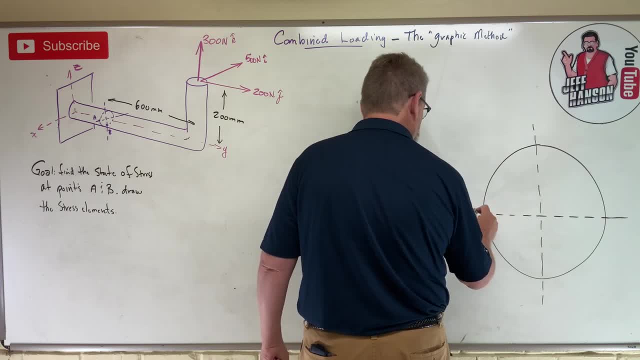 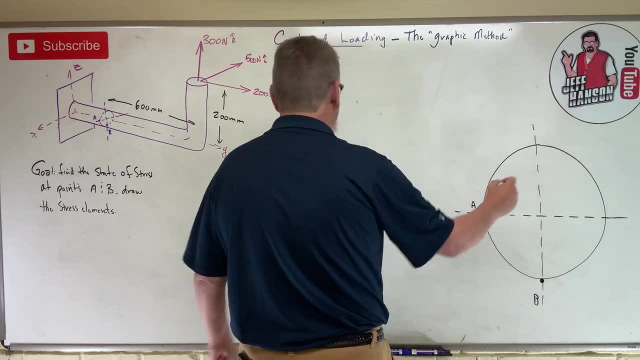 okay, point a is over here, there's point a, and where is point b? Point b is on the bottom, okay, So I drew this like I'm looking at it here. okay, There's my eyeball looking towards the origin. okay, And that's what I. 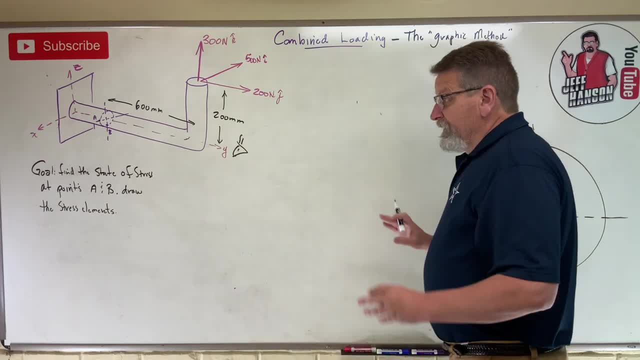 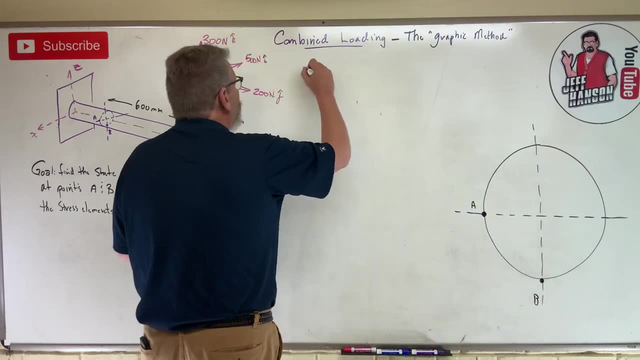 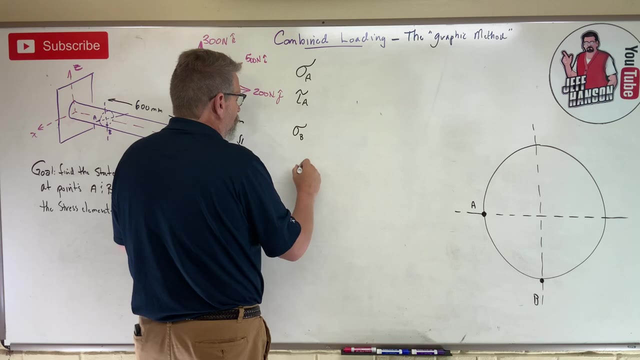 would see on that cross section. okay. Now the next thing I want to do is I'm going to go one force at a time, because what I'm going towards is this: I want to know what is normal stress on A, what is shear stress on A, what is normal stress on B? what is shear stress on B? right, I need. 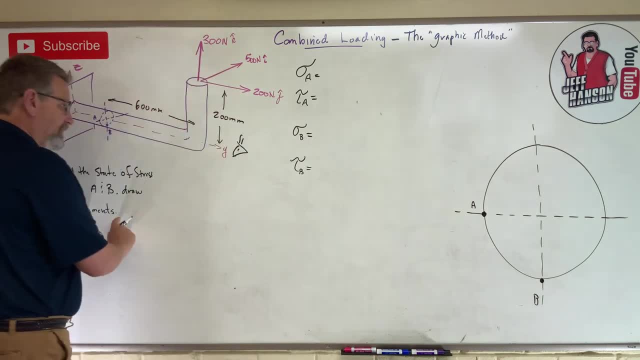 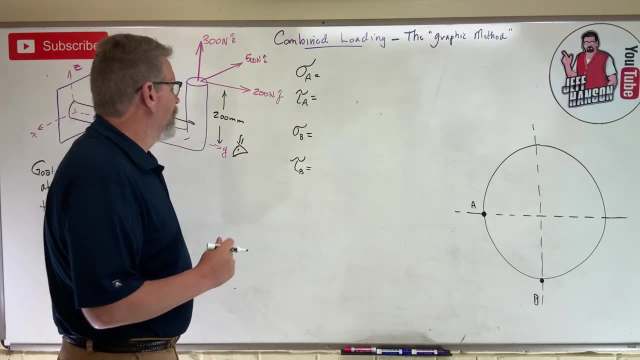 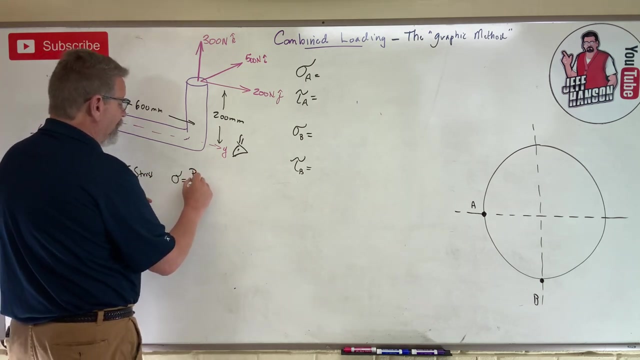 to know those things in order to construct my stress element, don't I? okay? So those are the things that I'm going towards. What's going to cause those things? Well, what can cause sigma stress? okay, Well, if it's a pressure vessel, I can have a little PR over T or a little PR over 2T. 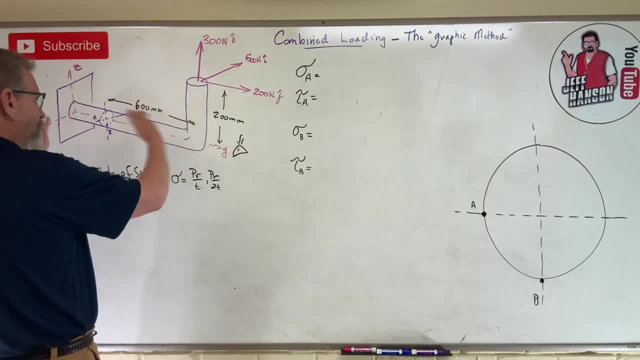 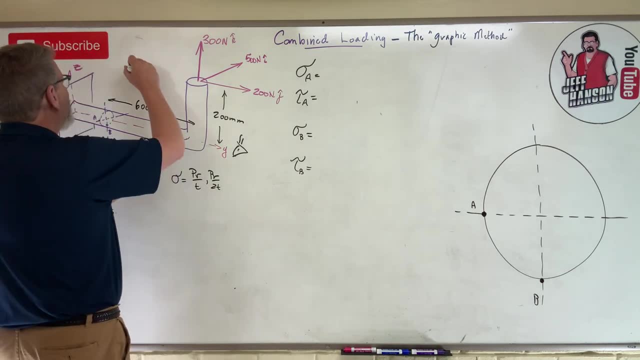 but this isn't a pressure vessel. This is some kind of solid steel bar here. okay, So I don't know about that. Let's give ourselves a diameter here. Let's say that the diameter of this bar is I don't know. 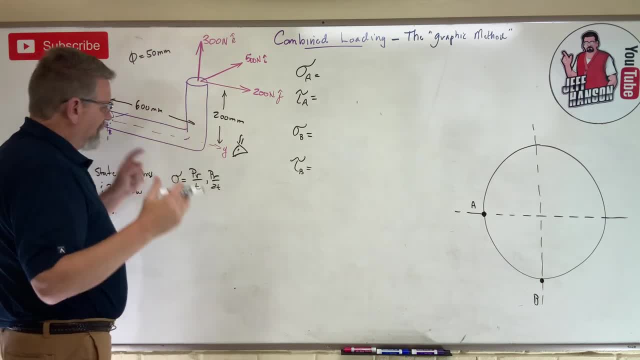 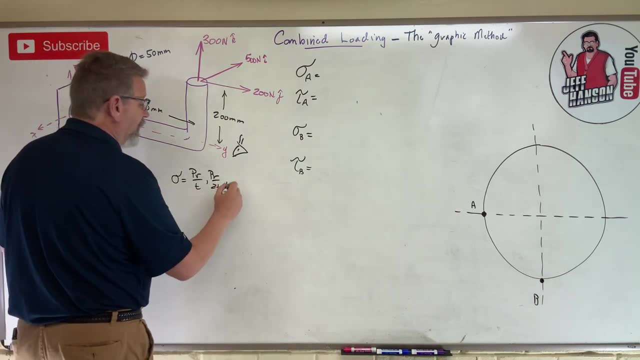 50 millimeters. okay, We're just making stuff up. so what the heck right? What else could cause sigma stress? Well, you know what? A little P over A, or, as I like to call it, not P, because P is confusing, I like to call it N- over A right, Normal force divided by the. 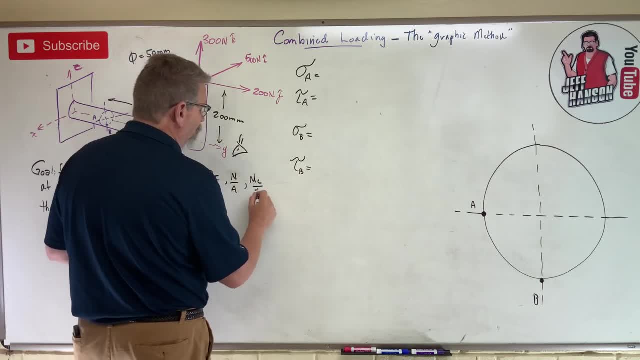 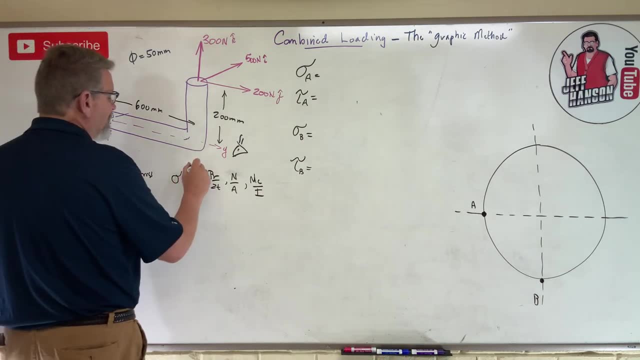 area, Normal force divided by the area, or a little MC over. I could do it, couldn't it? okay, A little beam bending. Those are the things that can cause stress. Now, this guy's out and that guy's out in. 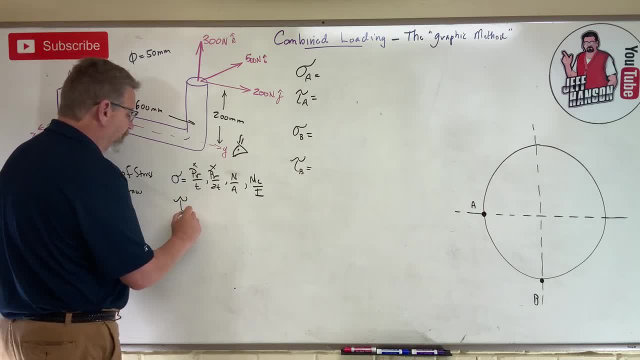 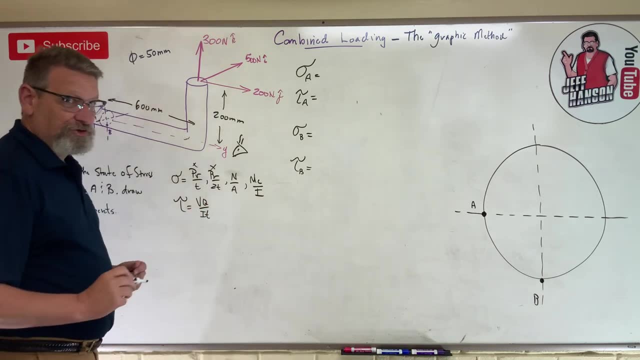 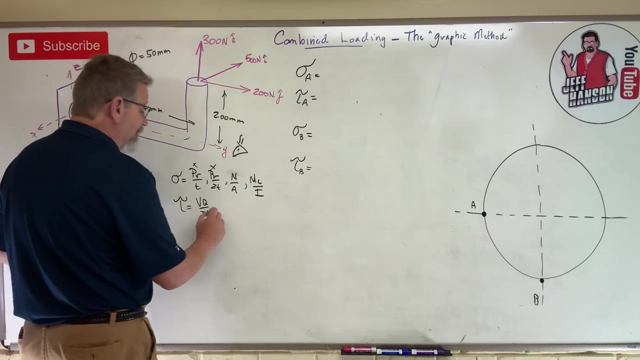 this problem. so I think we're just going to have these two guys. but what can cause some tau stress? Well, you can get that from a little VQ over IT right, which is just shear stress at a particular point and we are interested in a particular point, aren't we? okay So that? and then you can also 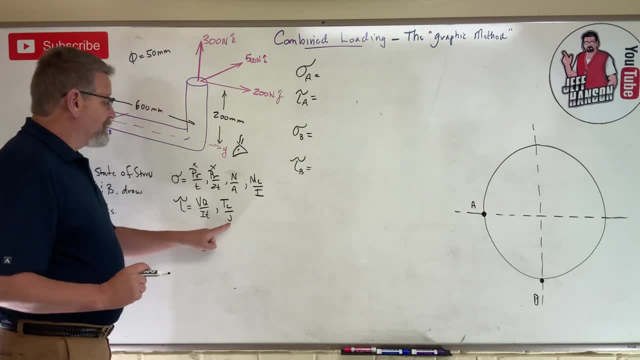 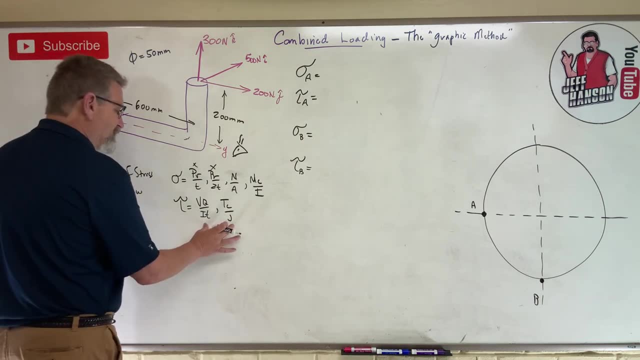 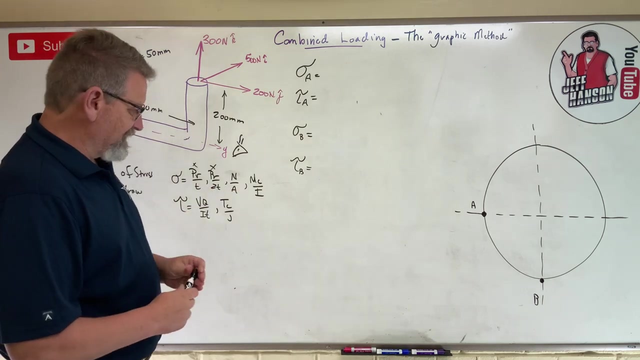 get shear from TC over J, which is shear stress due to torsion or twisting right. So I think that those are the two guys that we're after. We're after these two guys and those two guys, and we need the things that cause those things. okay, So what I'm going to do is this: This is what I call. 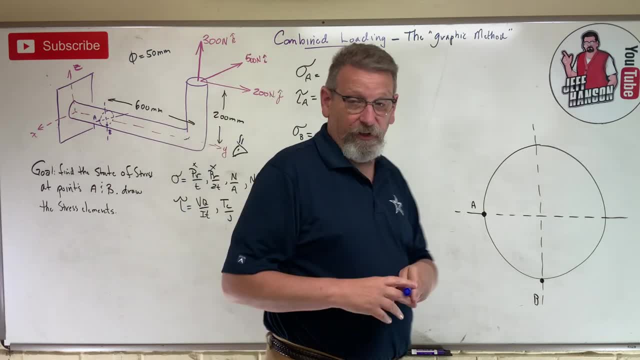 the graphic method. Call it what you want, That's what I call it. so here we go. I'm going to look at these three forces. Now I'll put an I hat, a J hat and a K hat to let you know that those forces 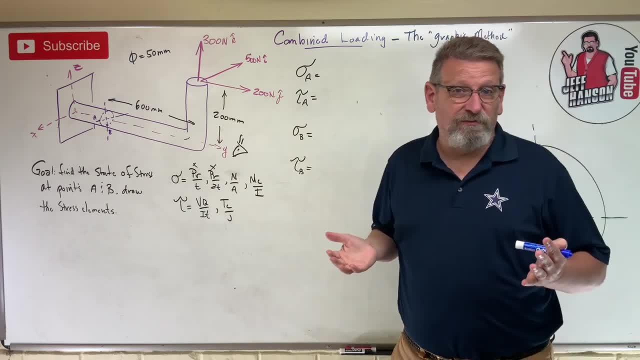 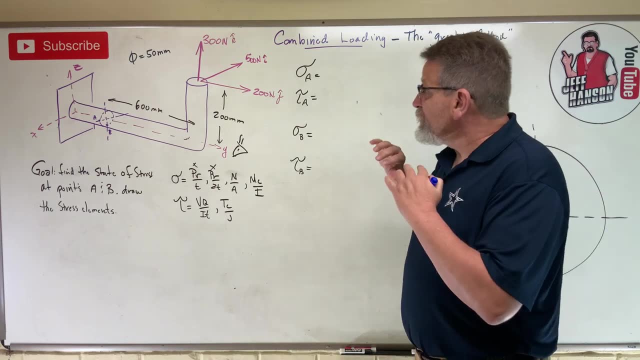 are along an axis. If they weren't along an axis, what would I do? I would just use trig and I would break them into components so that they were along an axis. right, So you can make any forces in the world into. Is Js and Ks right? We know how to do that from back at statics. We know that. That's. 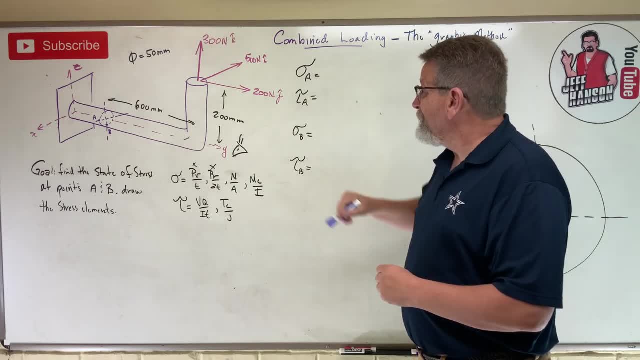 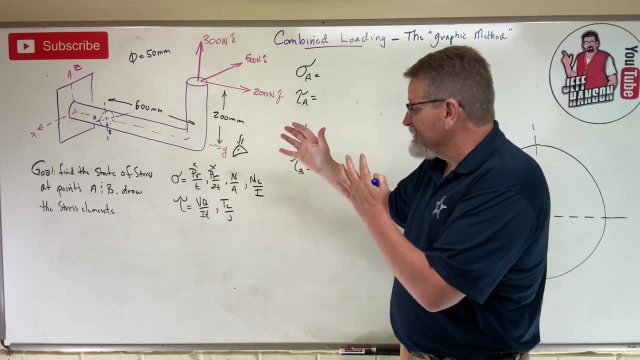 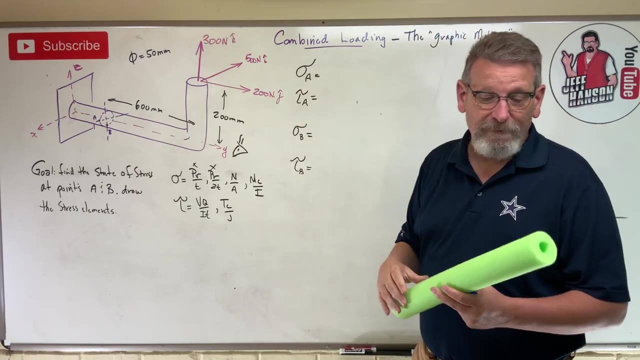 baby stuff. okay, Here we go. Let's do this. I'm going to go one force at a time and I want to know what on this system? what are the- let me get my noodle right- What are the effects of these forces? So I'm just going to start on the 200, okay, So what? 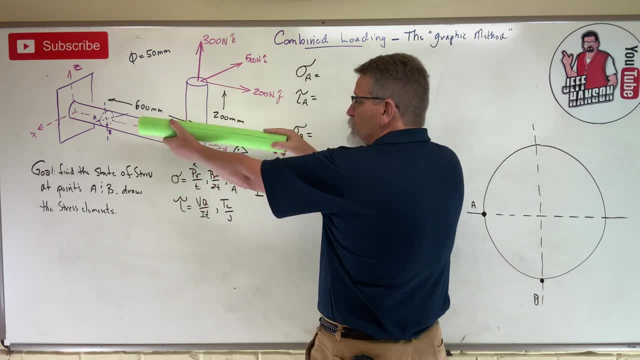 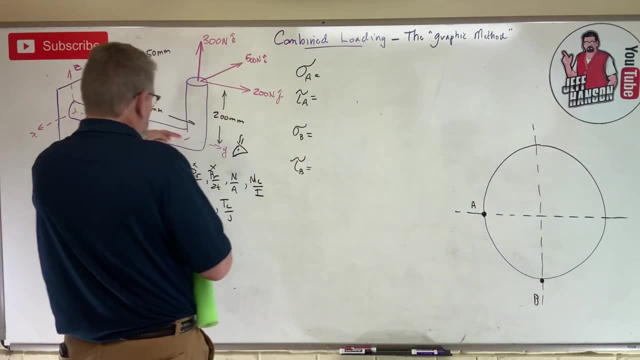 does the 200 do to me? okay, Well, number one, the 200 is stretching me, isn't it? Well, that's just causing an N, a normal force which is going in the Y direction. It's going along that axis. 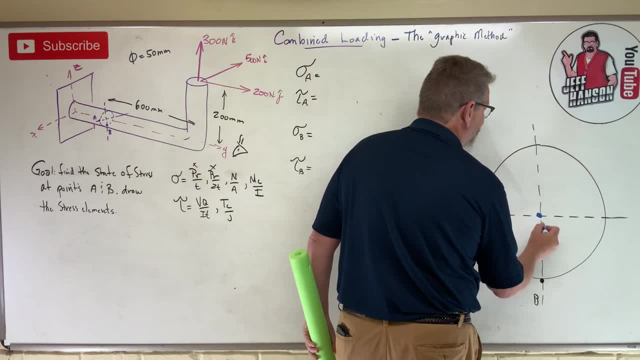 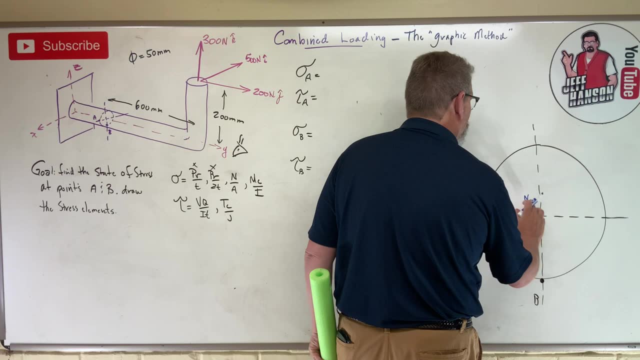 isn't it? So I'm just going to draw it as a dot. Why a dot? Because it's coming straight at you, isn't it Okay? So I'm going to call that N over A. Well, let's not call it N over A, Let's call. 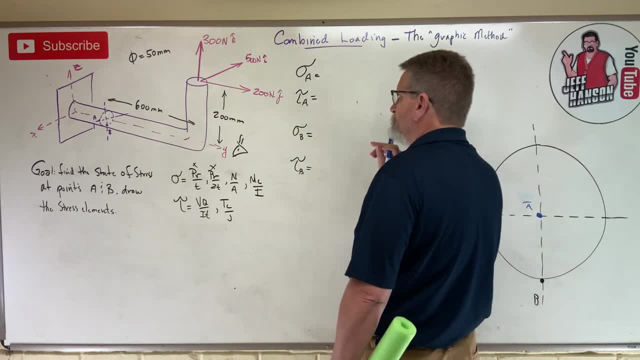 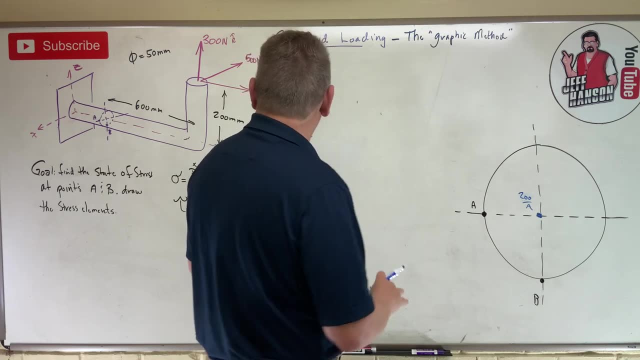 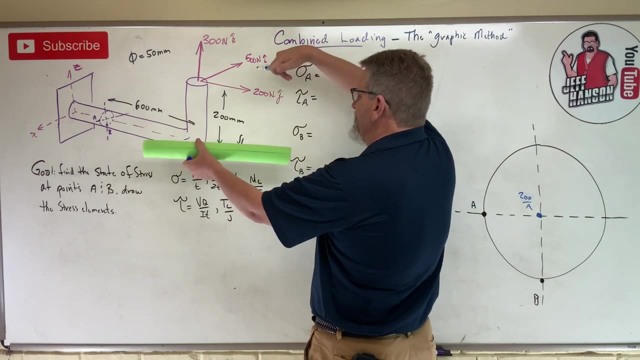 it. how big is that force? 200, okay, So I'm going to call it 200 over A. okay, There he is. okay. Does the 200 do anything else to me here? Oh, my goodness, Since the 200 is up here, right. 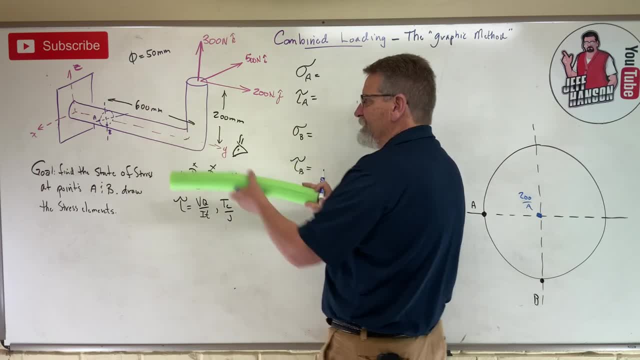 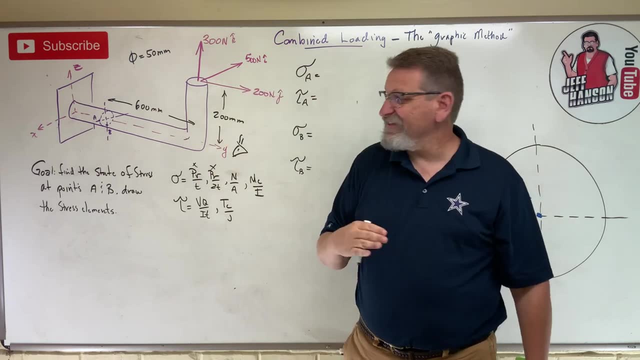 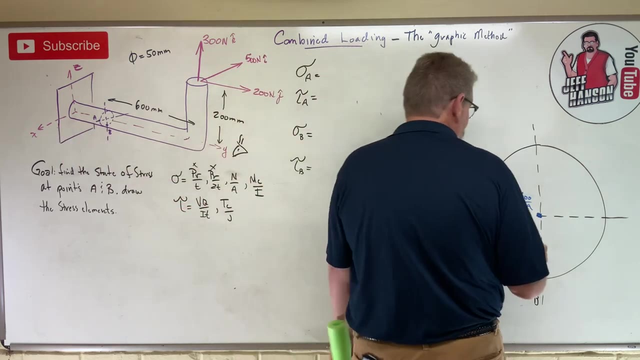 I think the 200 is causing me this bending right. It's causing me a bending this way, right, In this direction, around which axes? Around the X axis, isn't it Bending down around the X axis? So I'm going to draw that like this: 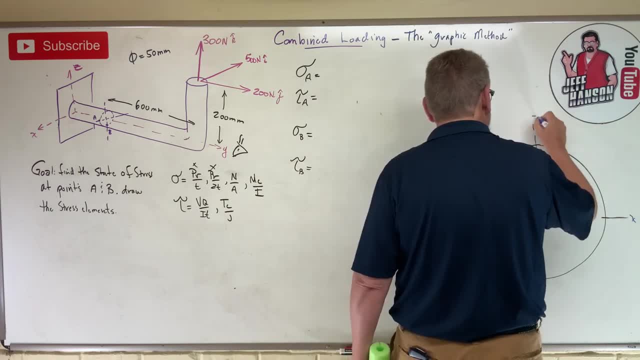 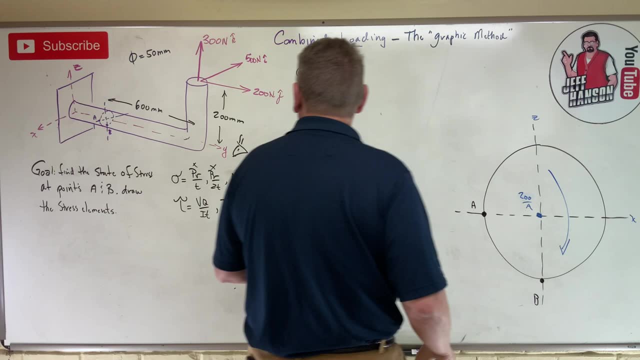 Here's my X axis, And this is the. this is actually the Z axis, isn't it? The Y is coming at you, So I'm getting this, okay, And how big is that moment? Oh, I'm going to show you a trick, This. 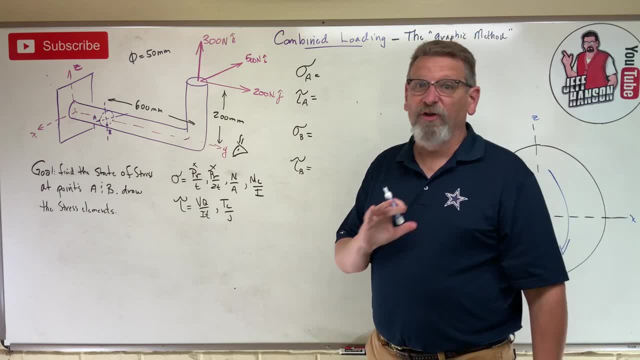 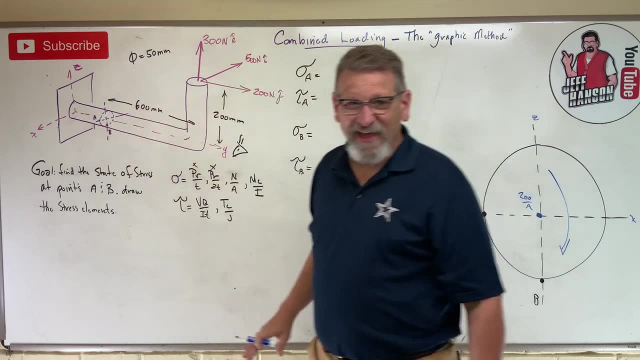 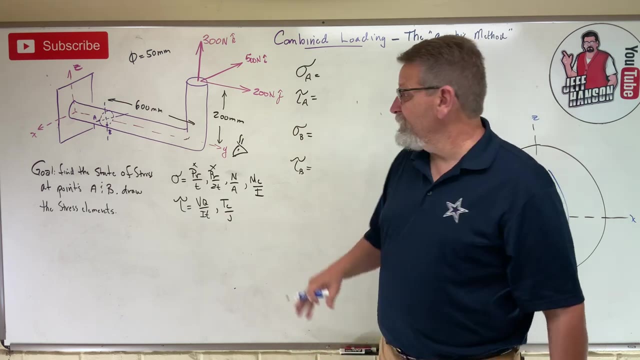 works every time. okay, Don't tell anybody else about this, This is only for the pros. okay, The force is in the Y, It's causing bending around the X, and so what's left? Z. Then the distance has to be in the Z. okay, So there's our distance. 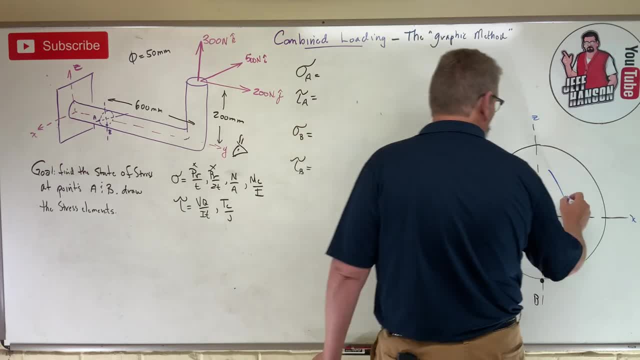 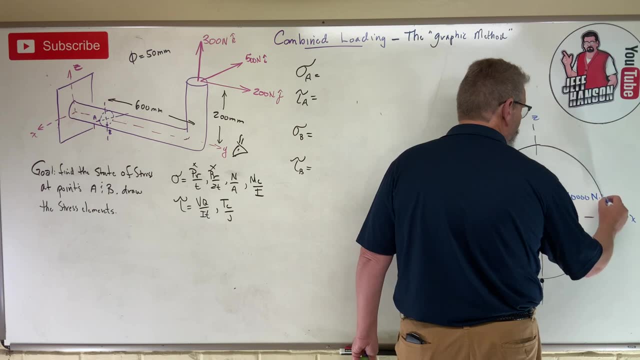 So it's 200 times 200, right? So that's 4 with 1,, 2,, 3,, 4 zeros, and that's going to be what? Newton millimeters, okay, So I think that's all the effect. Now, again, what do we have over here? 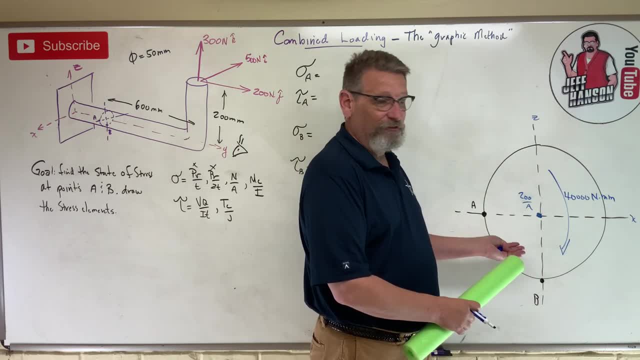 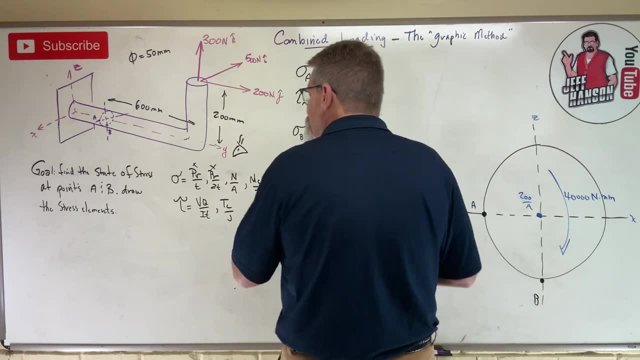 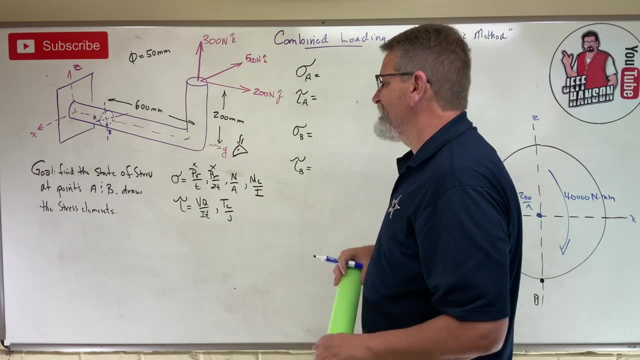 This is the sum of the forces or the moments around an axis. really, I'm drawing those graphical effects of each one of those forces. okay, It just helps me to see that picture better. I think that's all the 200 causes, okay, So let's move over to the 500.. What does? 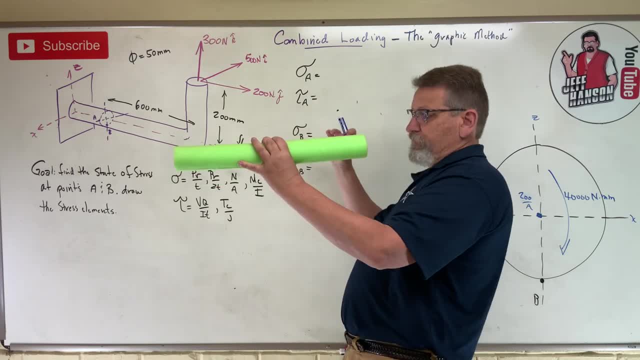 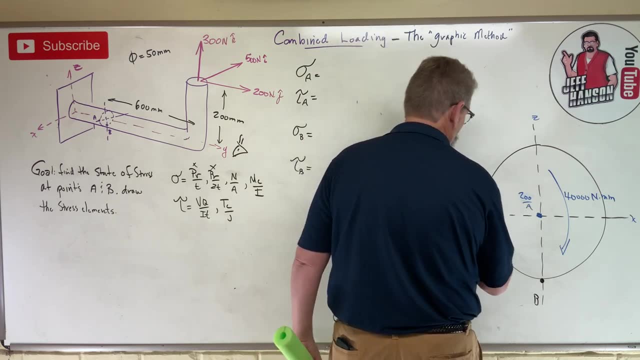 he cause: Okay, the 500 is just trying to just tear me to the side there. okay, Which is a V force, and I'm going to draw that like this. So V equals 500 newtons. There's my shear force, okay. 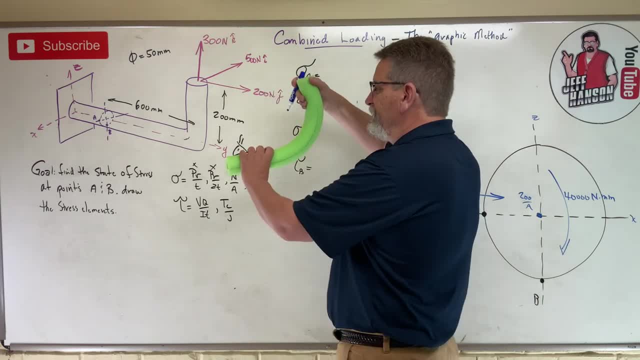 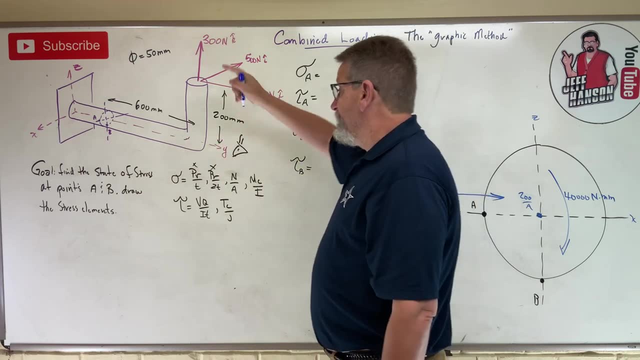 So he's causing a little shear. What else is he doing? Well, since he's up here, he's causing a right, He's causing a rotation, He's causing a torque right And it's trying to rotate around. 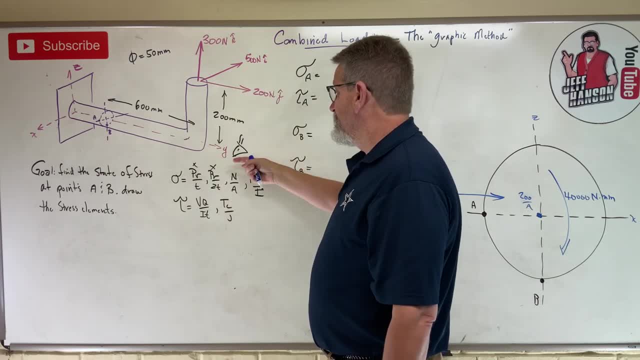 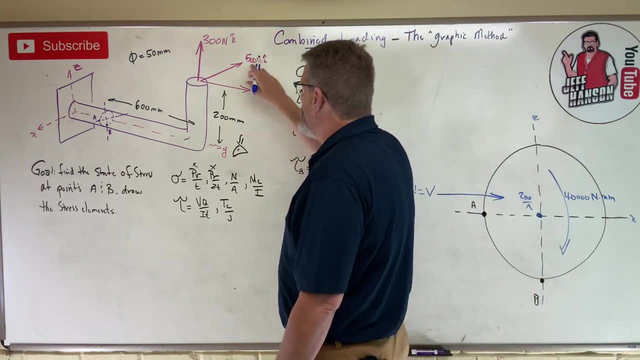 that Y axis, isn't it? The force is in the X, It rotates around the Y, so the distance is in the Z. It works every time okay. So 500 times 200 is creating a torque. Now I'm going to draw that. 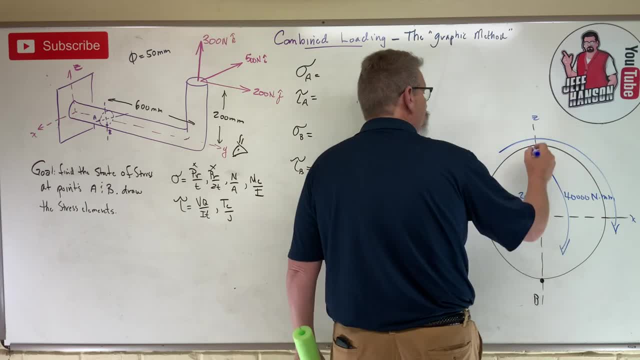 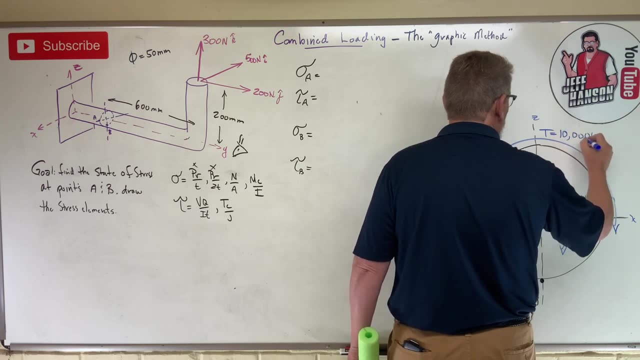 torque like this. okay, So T equals 500 newtons. What 500 times 200 is 10, with 1,, 2,, 3, 4 zeros, That many, and that again that's newton. 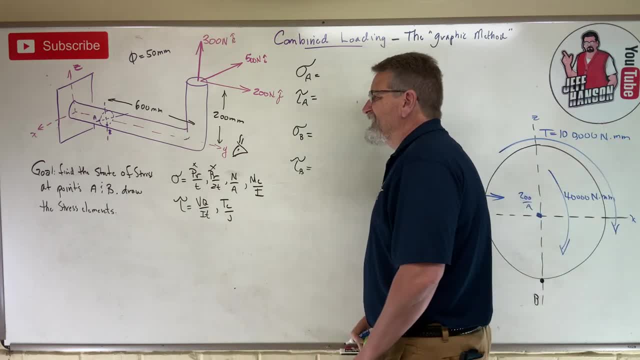 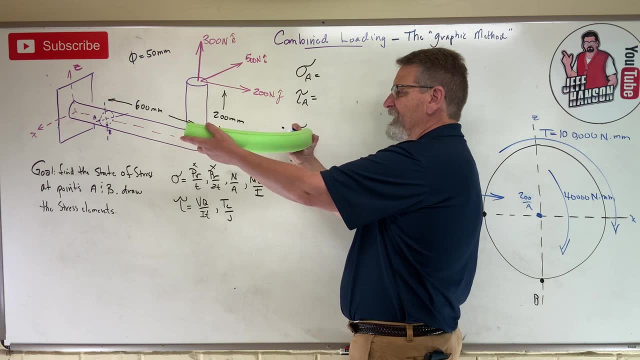 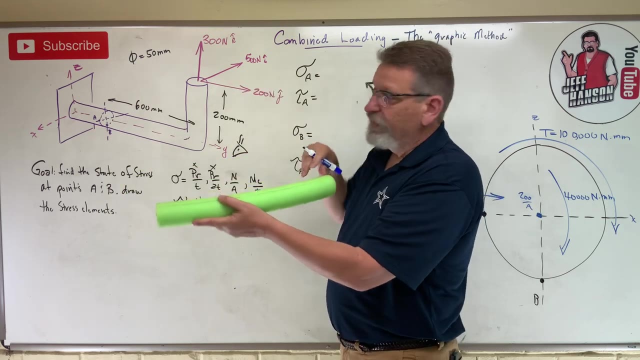 millimeters, okay. Does he cause anything else? You know what He does, doesn't he That 500 also just causes a bending like that, doesn't it? Okay? Around which axis? Which axis is that causing a bending? Around the Z axis, okay. So the forces. 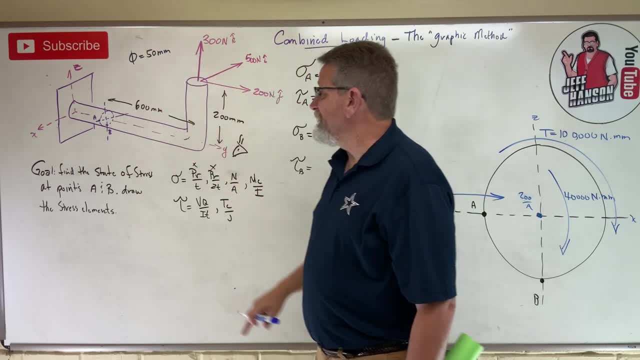 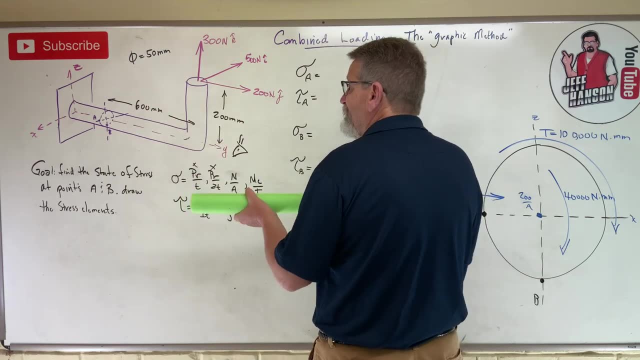 isn't it The X? it bends around the Z, so the distance is in the works every time. Okay, so six times. so that's causing a bending around the Z like this. I'm going to draw it like that. 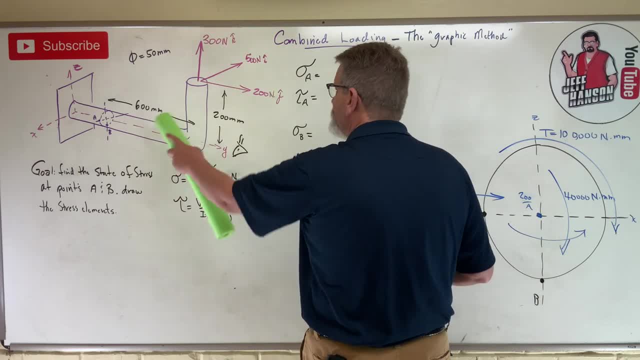 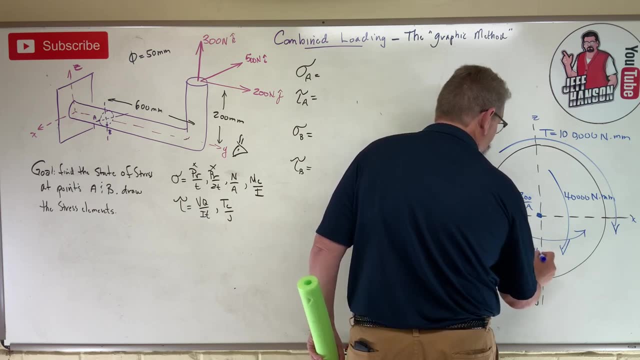 okay, And I'm going to call that 500 times 600.. That's 30 with 1, 2, 3, 4 zeros on it and that is newton millimeters. okay, I think that's got the 500.. So 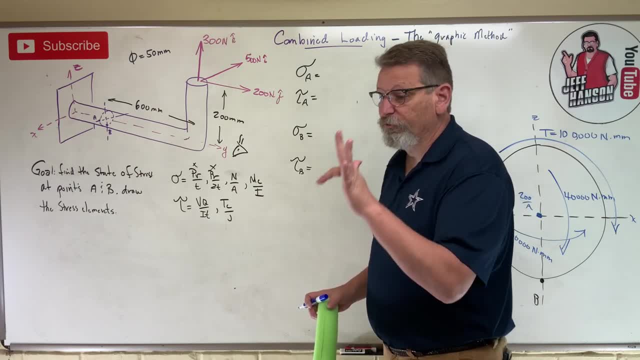 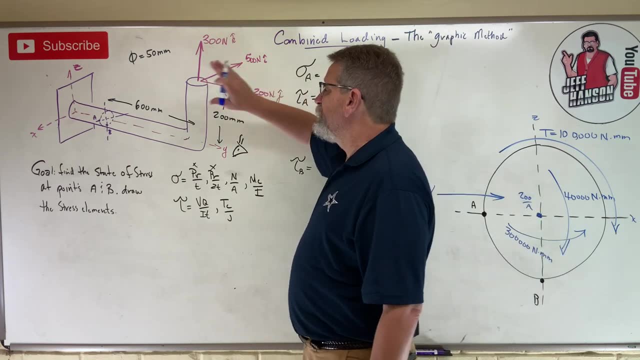 you know, one force can do a lot of things. It can cause bending, it can cause torque and it can cause a force, a shear or a normal force. right, All right. last guy, the 300.. What does he cause me? okay, Does he only causes a shear, doesn't he Just trying to tear straight? 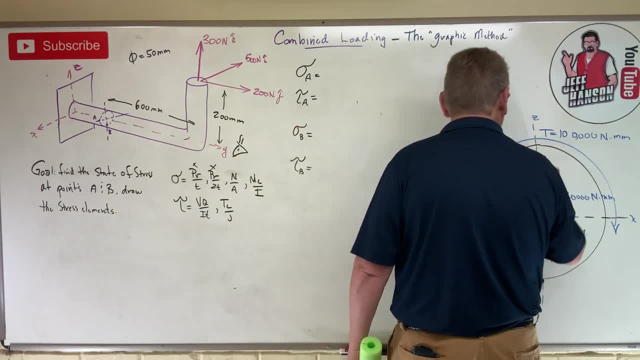 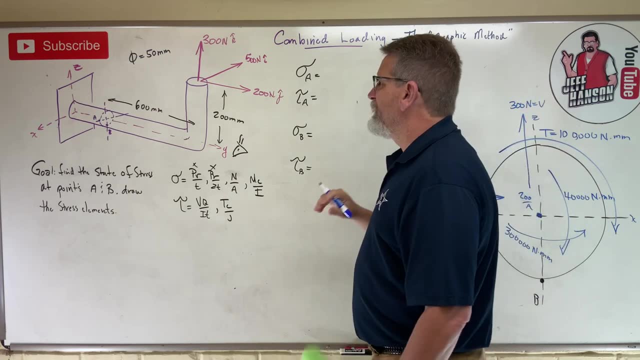 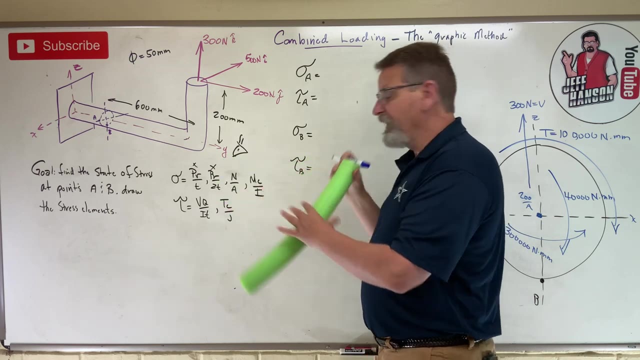 upwards right. So 300 straight upwards, whoop. okay, Equals V, there you go. And then what else is he doing? It's causing bending on my beam like that, isn't it? That's bending around the what Around the X, right? 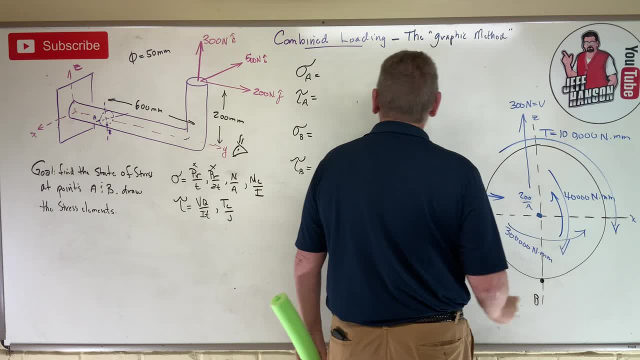 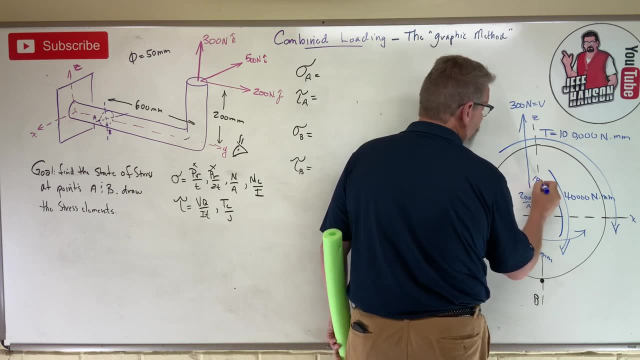 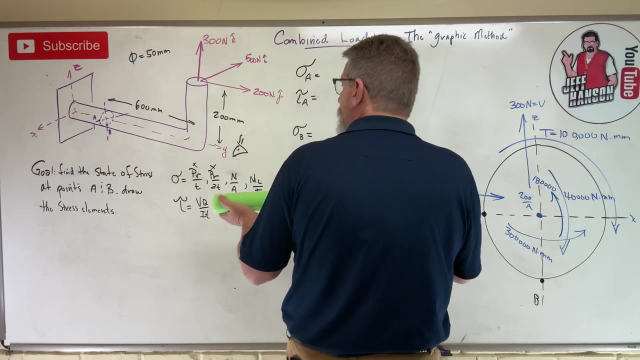 Upwards though. So like this: And how big is that? 300 times what? 600, right, So that's 18 with 1,, 2,, 3, 4 zeros. okay, And so I think that's all I get right Of shear force. 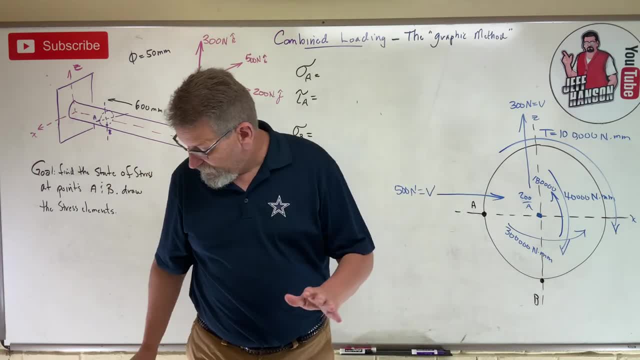 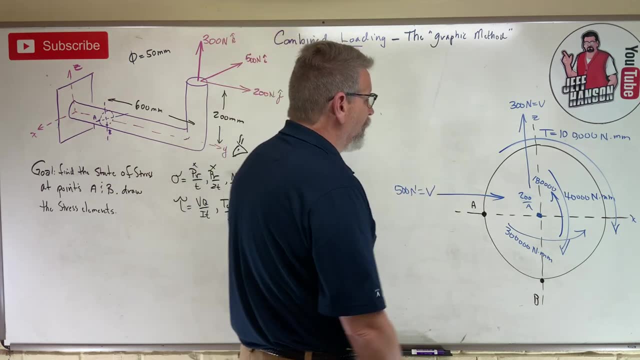 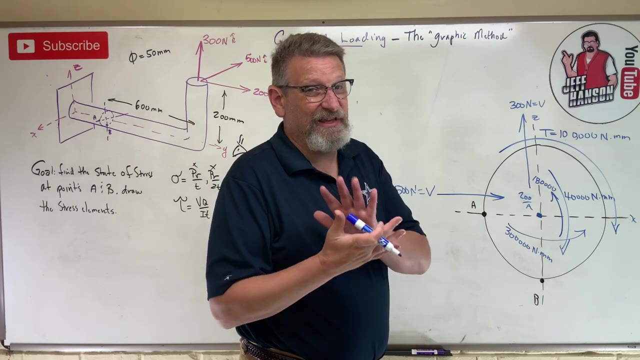 yeah, that's it. So there it is. Now, once I get it to this state, I want to simplify that, right? Can I simplify that? Well, look here, moments around the X, I got one up and I got one down. I can add those together and get them together to get a net. 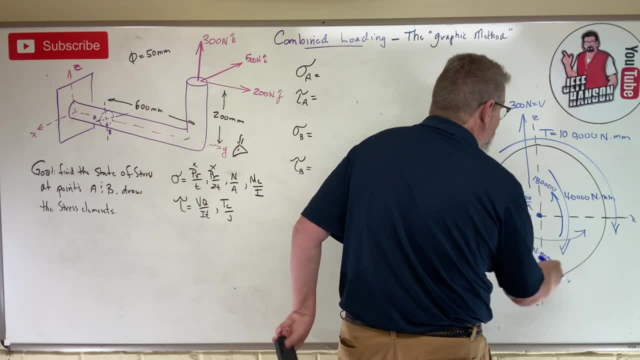 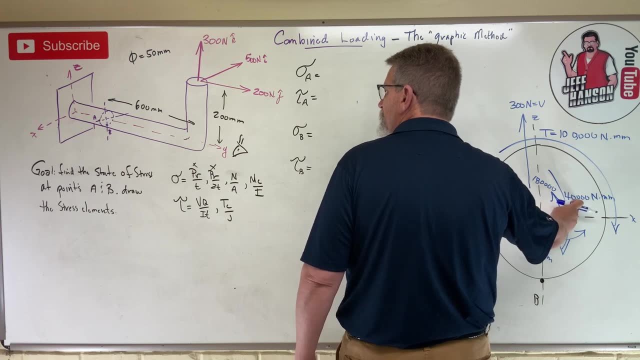 moment. So I got, I got what 40,000 down. Where's that 40,000 come from? That was from the 200 times 200.. 1,, 2,, 3,, 4, yeah, okay, And I got 180,000 up and down. I got 180,000 down, I got. 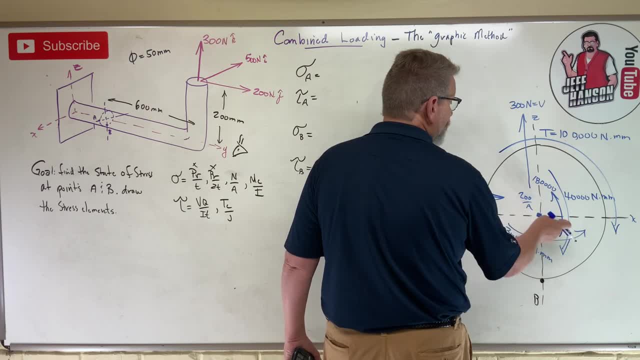 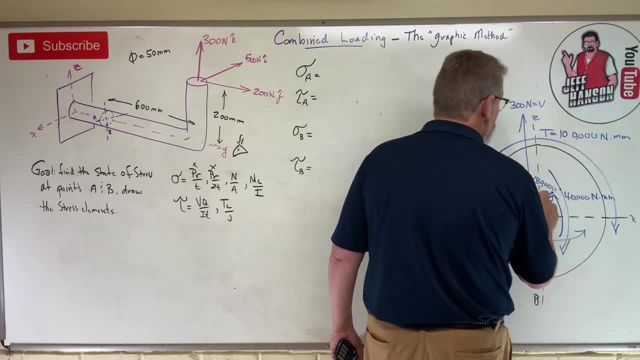 180,000 upwards. So, yeah, that's going to this. one's going to win, isn't it? So 180,000 minus 40,000 is 140,000, isn't it? So what I'm going to do is I'm just going to get rid of this guy. 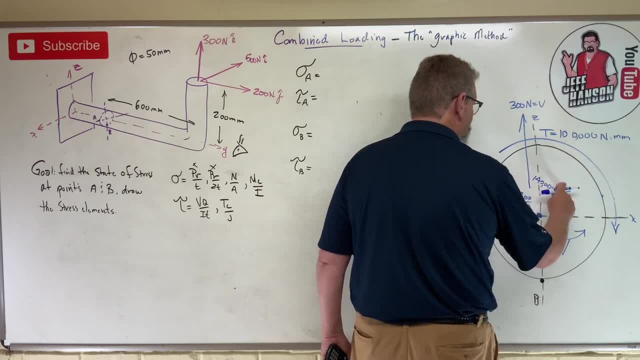 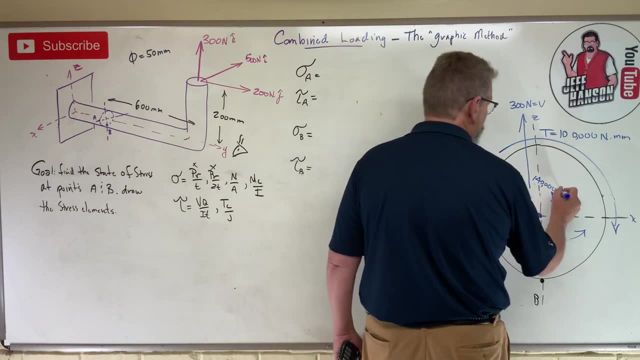 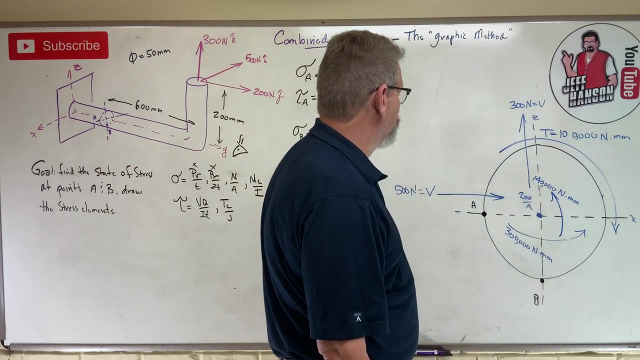 okay, Because I combined those two together, right? So I'm going to get rid of that guy all together, okay? And that's newton millimeters, okay, Now what, That makes it a little simpler, right? Well, now I'm going to come over here and I'm 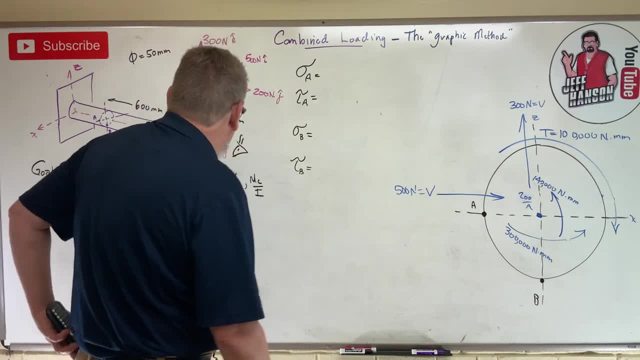 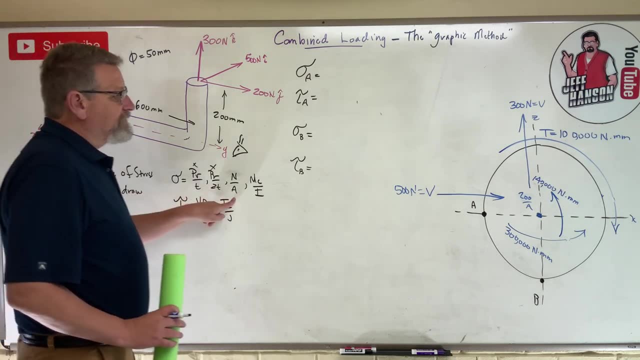 going to say, okay, let's go, Point A. okay, Sigma A. Oh, where'd my noodle go For sigma A? what am I doing? I'm doing? is there an N over A? Well, yeah, there is There. he is right there. 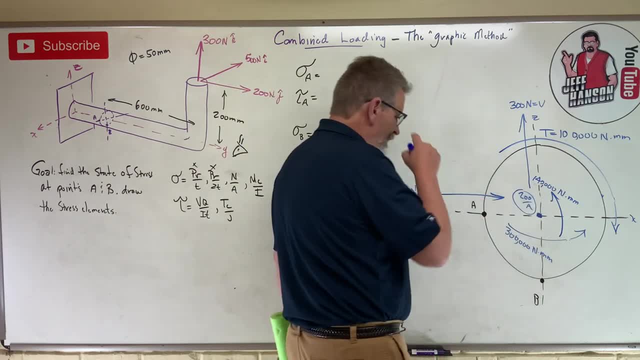 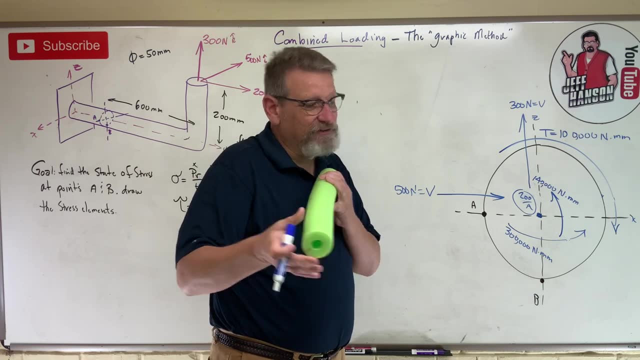 I'm going to take care of this guy all at once. okay, He's stretching. So for point A and for B, they're both going to be in tension. Tension what Starts with a T, which is a positive sign. 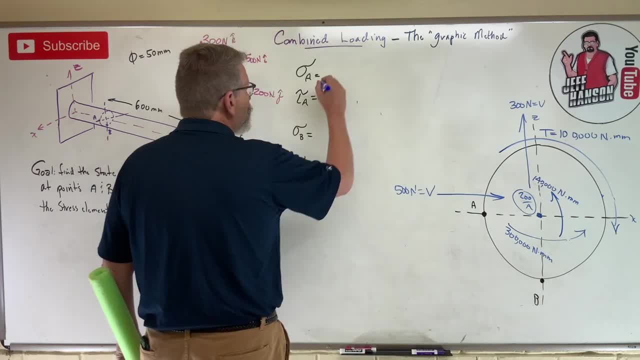 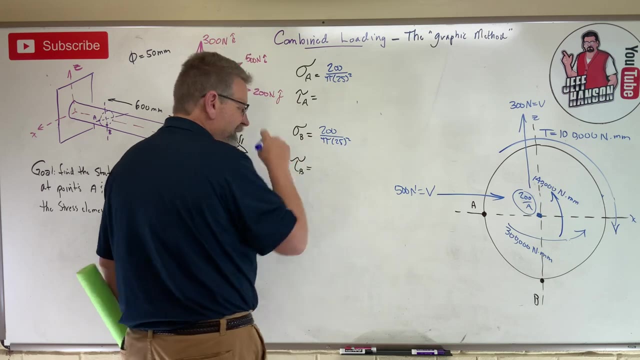 right. So I'm going to get a plus 200 divided by A, which is pi times R, squared, right? And I'm going to get it for this guy too: 200 divided by pi R squared, okay. So that's got that guy. 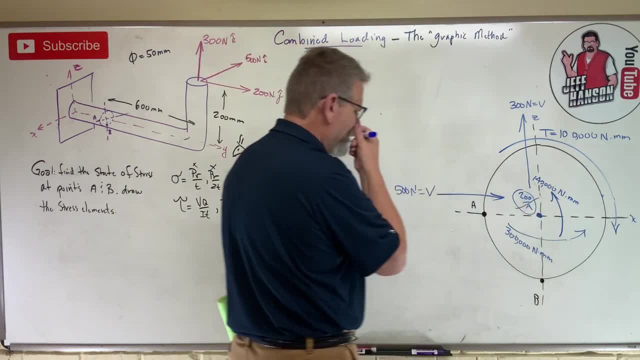 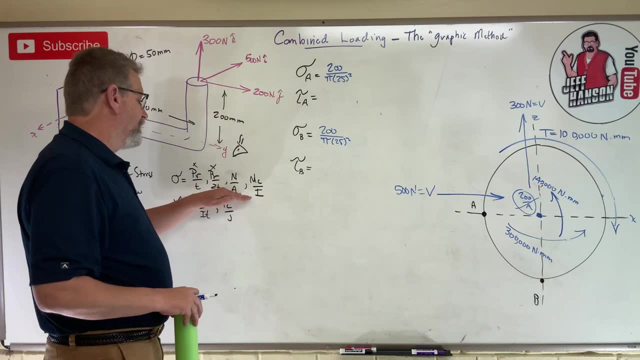 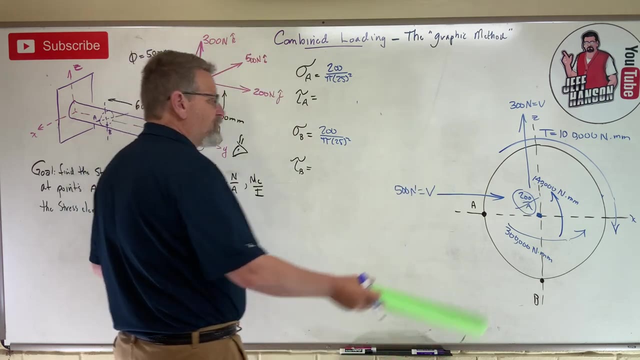 taken care of Check We got him. Does V cause any kind of normal stress? No, So that's gone, That's gone. Does torsion cause normal stress? No, So, only these two bending moments are left right. 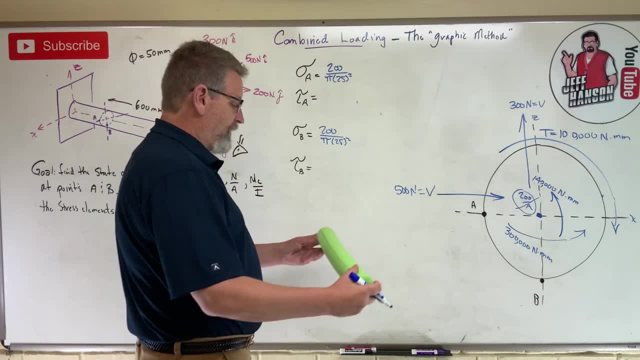 Okay, So here we go. Now, this is where your noodle's going to come in handy. I'm going to put my line over here at A and the 140, right, Which is bending this way? I'm going to bend it. 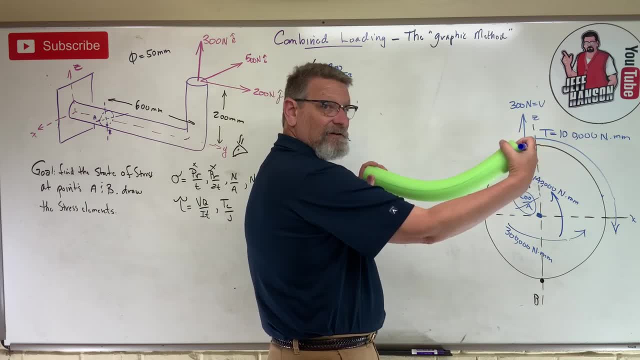 like that. So A is going to come in handy. I'm going to put my line over here at A and the 140, A is over on this side. What do I see? Point A is on the neutral axis, isn't it For this? 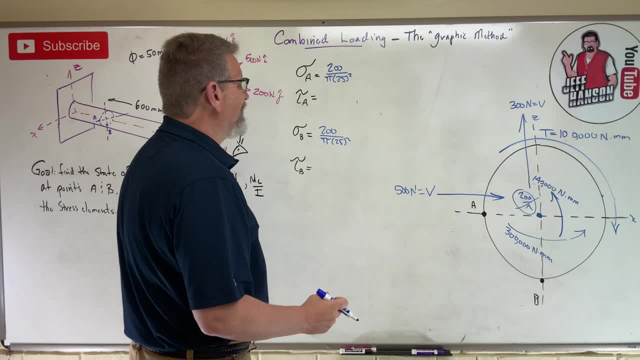 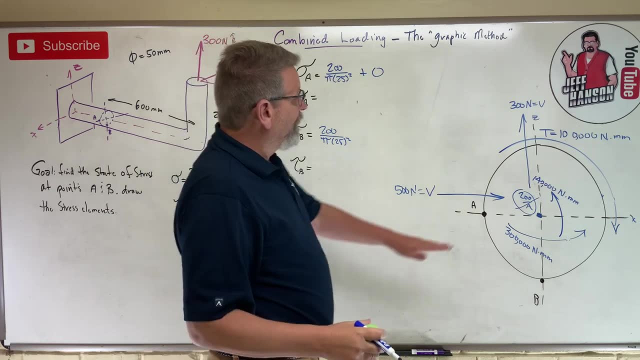 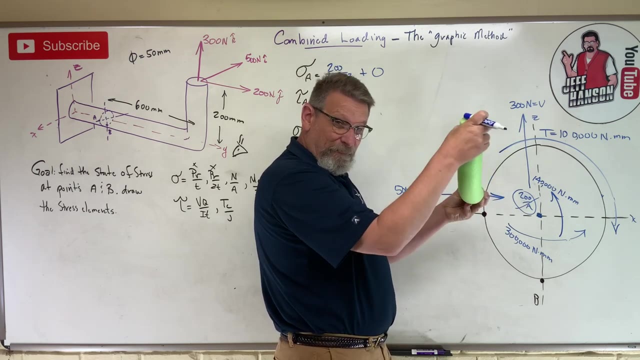 for the 140, right? So if it's on the neutral axis, what does that mean? There is no normal stress from that guy. okay, Now the 140 is bending up. Where does point B live? Point B lives on the bottom of the part, So point B is in what Tension? right? So let's get the point B down. 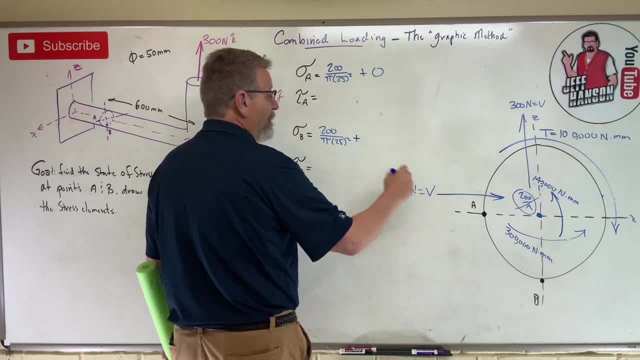 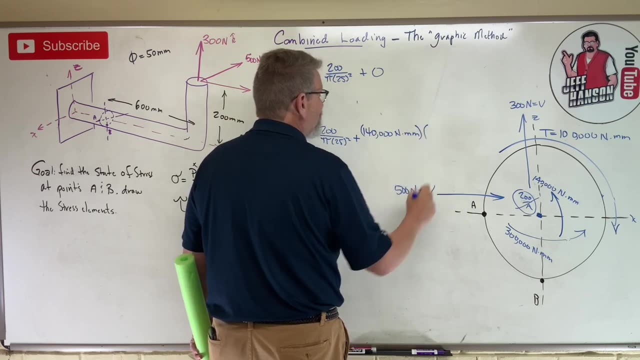 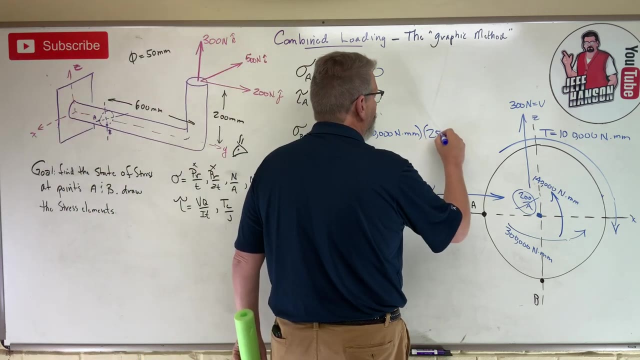 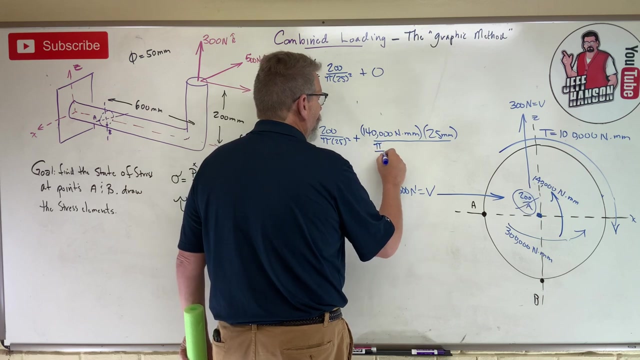 here, which is a plus, And we've got MC over I. M is 140,000 newton millimeters, right. What is C? The distance from the neutral axis to the outside of the part, which is 25.. And then what is I for a round part? Well, it's pi over 4R to the fourth millimeter. 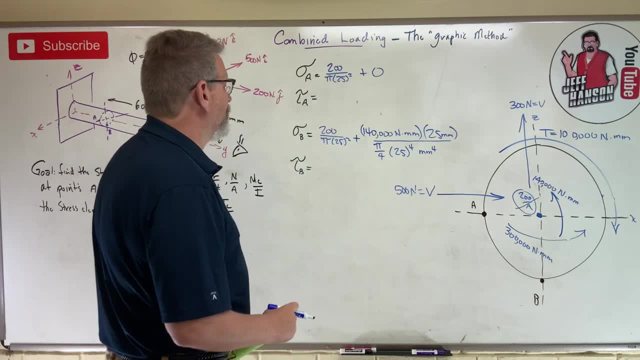 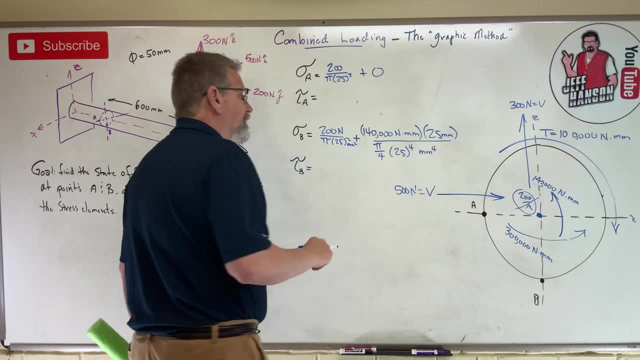 So there's our number for that. right Now, this guy was in newtons and then this guy's in millimeter squared, MM squared. okay, All right, And so this one's going to be in newtons and 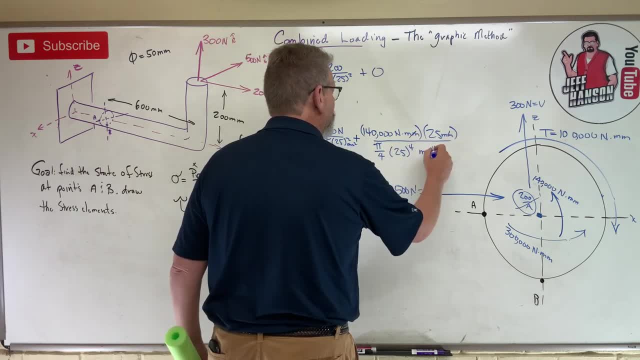 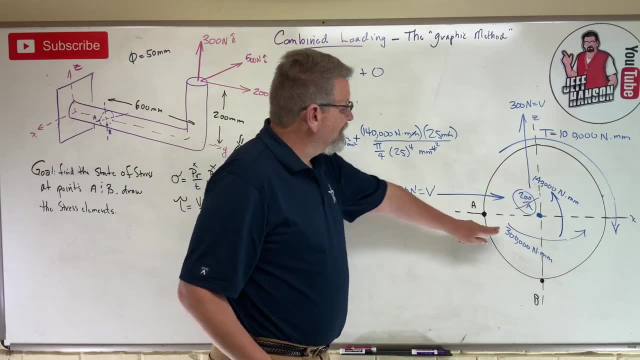 there's an MM and an MM. This is going to be millimeter squared also, isn't it? Okay, That's good stuff. So we got that guy right. Check, Let's get this guy. okay, He is bending Here's. 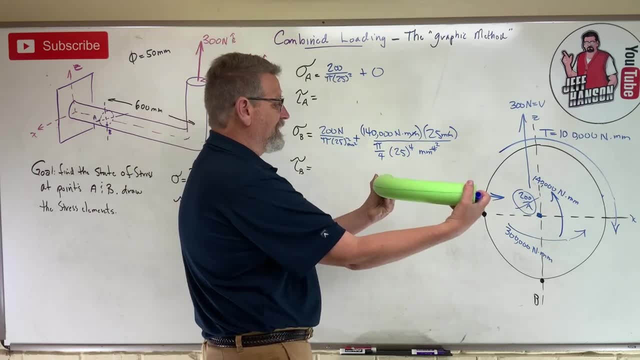 my line down my beam. He's bending this way, and he's bending this way, and he's bending this way, isn't he Okay? So what's he doing? So for point A, point A lives on this side over here. 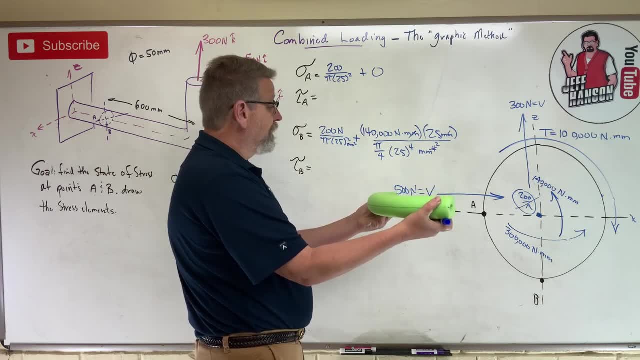 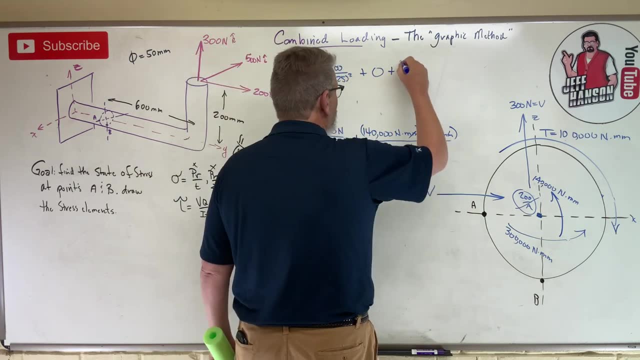 right. Point A is going to be what Well? it's in tension, isn't it? So point A is going to be in tension, So he's a plus. The size is 300,000, right, Same as this times: C 25,. 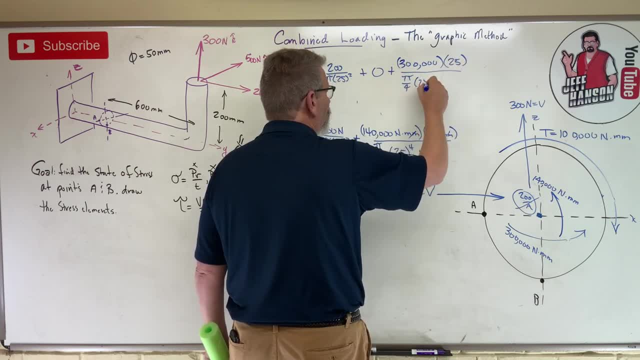 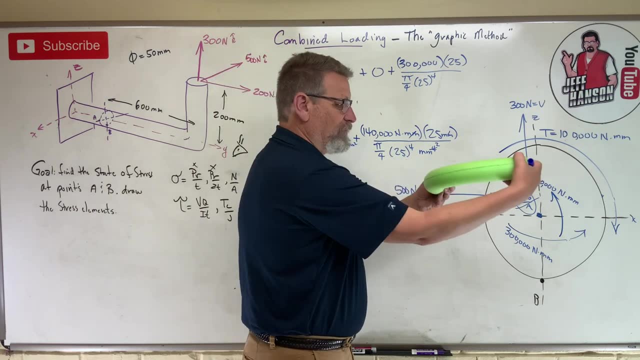 divided by I pi over 4R to the fourth right. That gets me to the other side right. So it's that guy. And then what about this one? What about B? If I'm bending this way, where's point B? 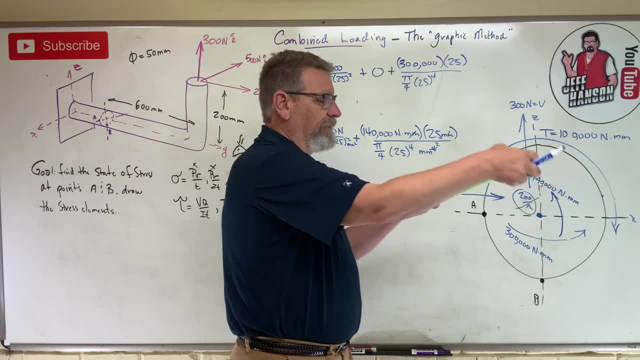 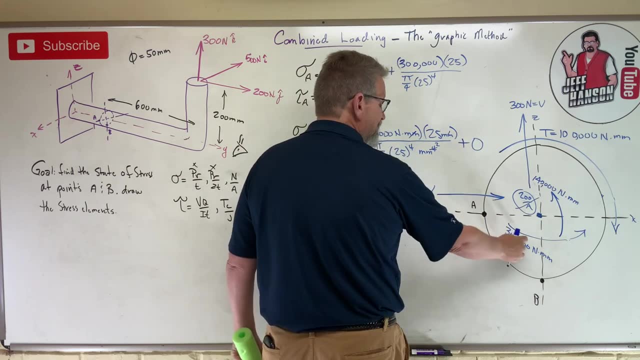 He's on the very bottom of the part. Let's see Here he is right. Where is he on the bottom of the part? Oh, he's on the neutral axis again, isn't he? So for point B, it's zero from the 300,000,. 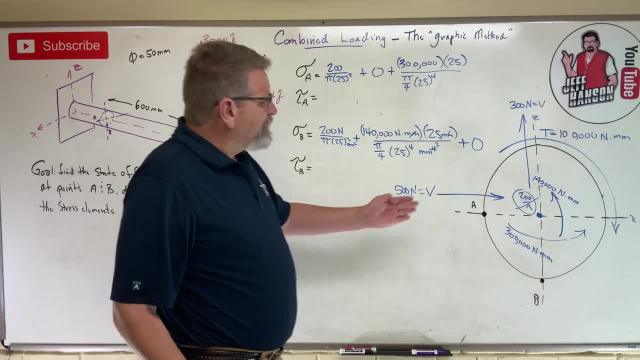 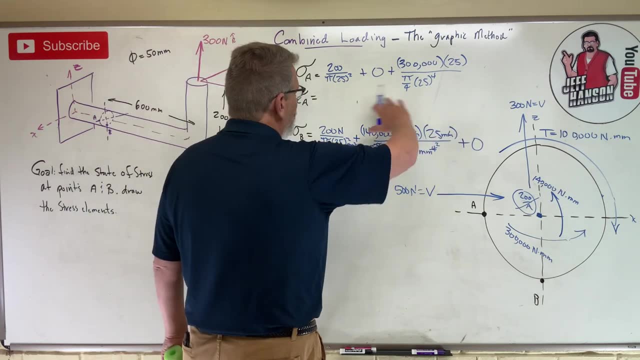 okay, So just going one force at a time across my graphic of the cross-section. there I got it, man. I got to put this in my calculator, But I got it. So we'll do that here in a second. We'll get those two guys. 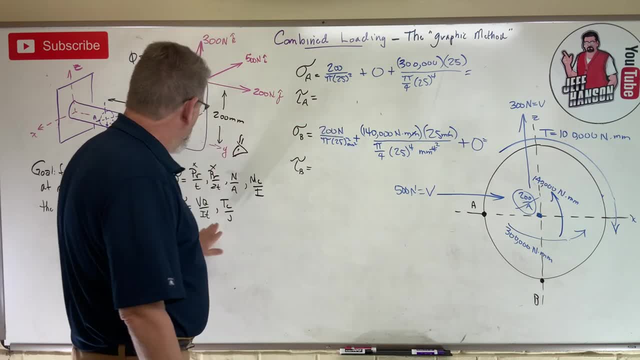 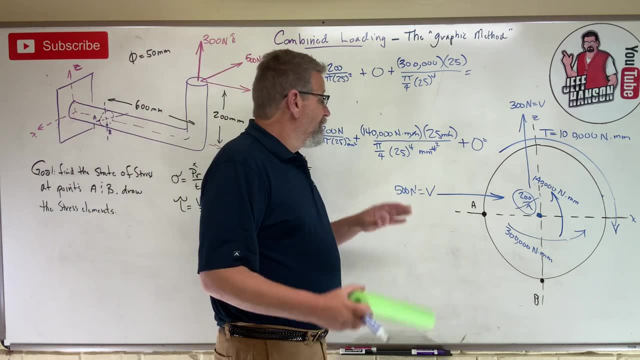 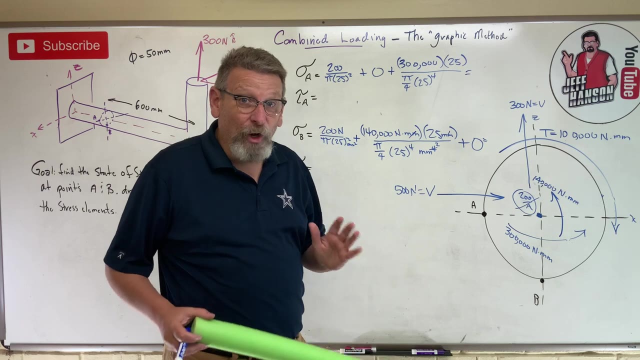 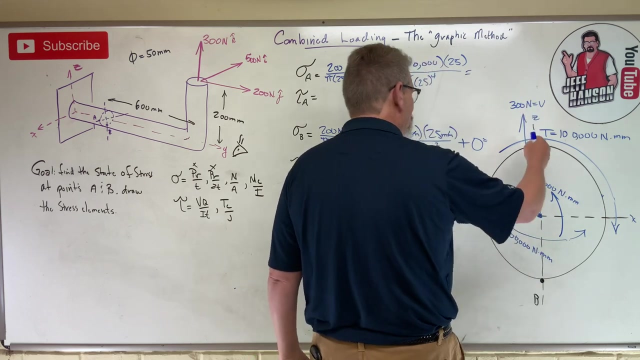 Let's talk about tau. What's going to cause tau? okay, VQ over IT. Let's do VQ over IT first. okay, Can you answer this question? The neutral axis is always blank to the V force Perpendicular right. So if V is pushing this way, the neutral axis is this way. If V is pushing, 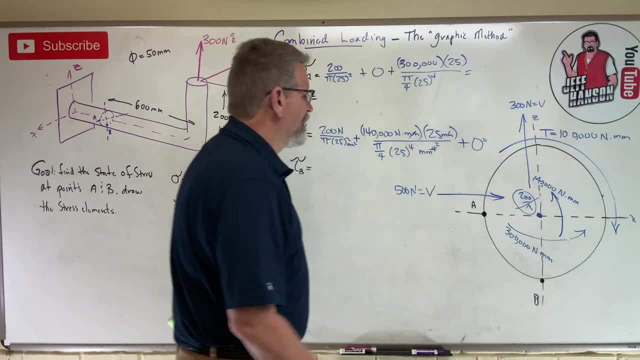 this way, the neutral axis is this way. If V is pushing this way, the neutral axis is this way. The neutral axis is this way, right, Okay? So let's start with the 500,. okay, The 500 pushing. 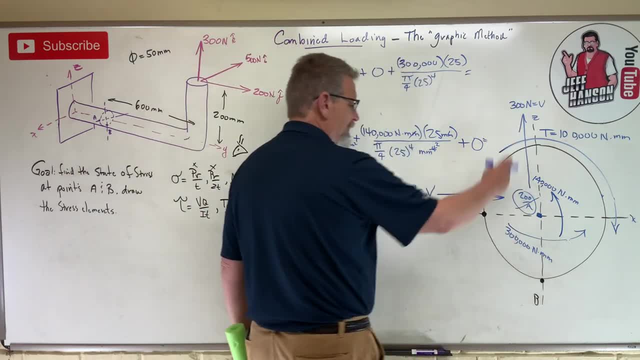 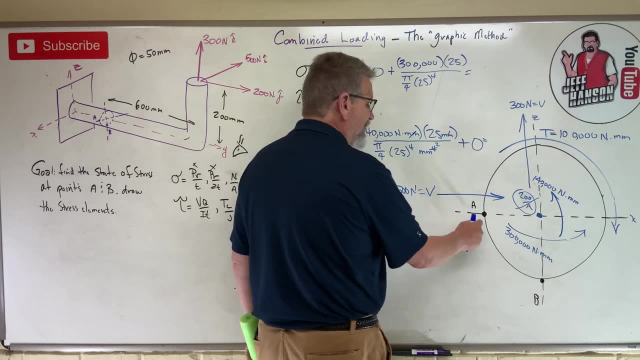 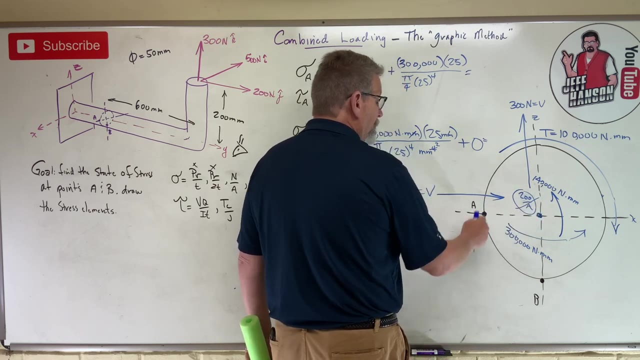 this way, which means the neutral axis is up and down right. It's in the Z direction, which means that point A right At point A, what's going to be Q for point A, for this 500, right? Well, point A is on the very outside of the part. How much area is above? 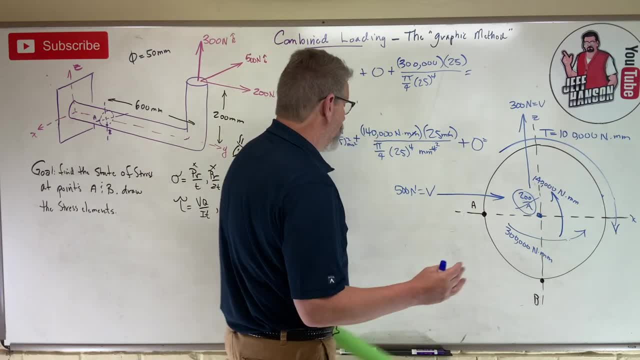 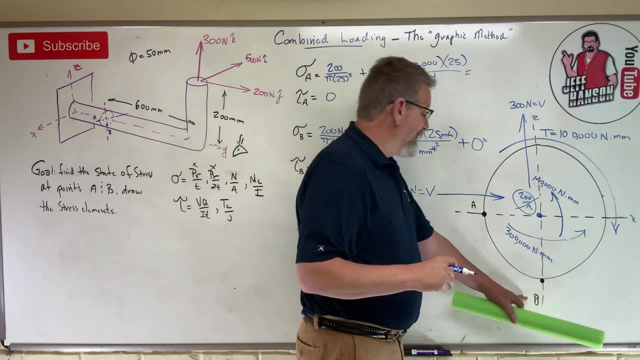 point A: Zero. So for the 500, point A is going to be zero right Now. for the 500, point B, no, What's Q going to be for point B? Okay, Here's the neutral axis. Point B is on the neutral axis. 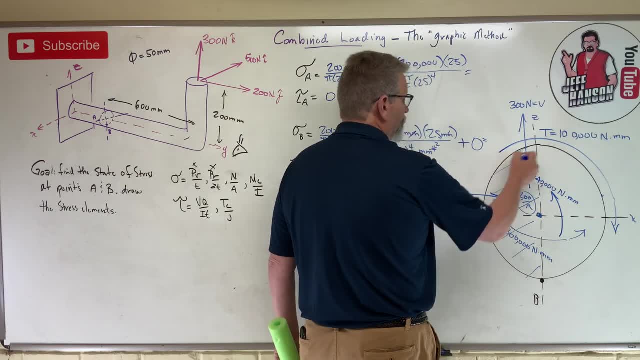 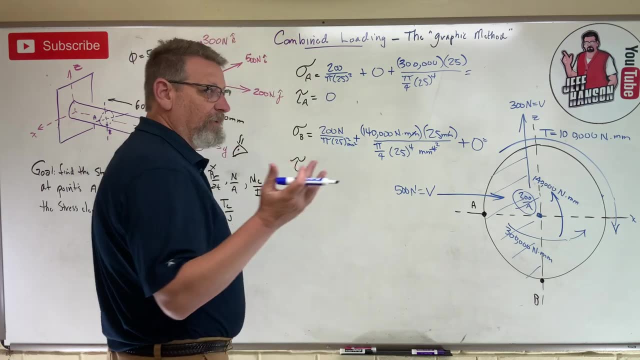 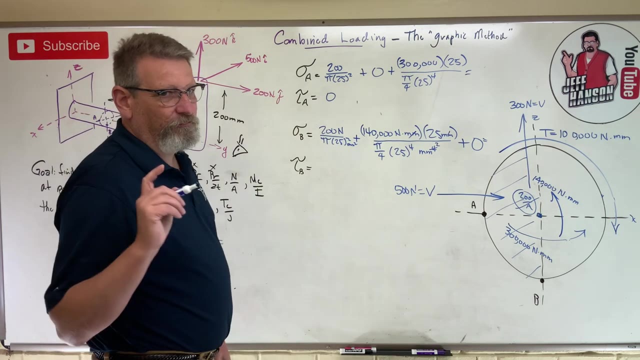 which means Q is going to be all of that. right, I thought it was going to be all of that over there. It's the same thing, okay, And remember this. Do you remember the shortcut for Q? Do you remember? So Q is Y bar times A. What's Y? bar for half a circle, Four R over three pi, What's A for half? 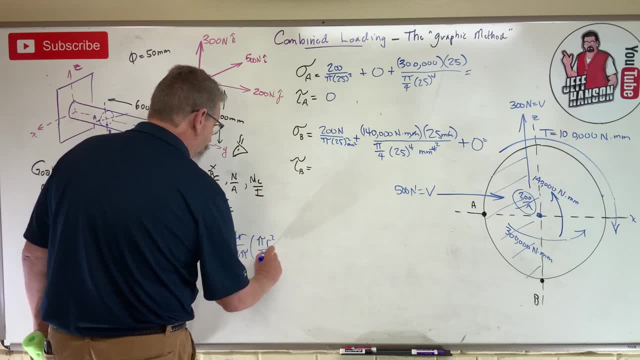 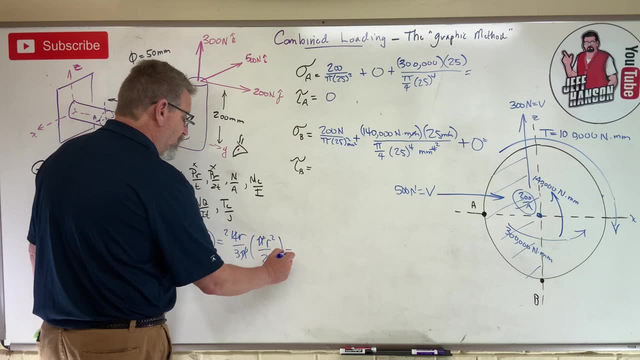 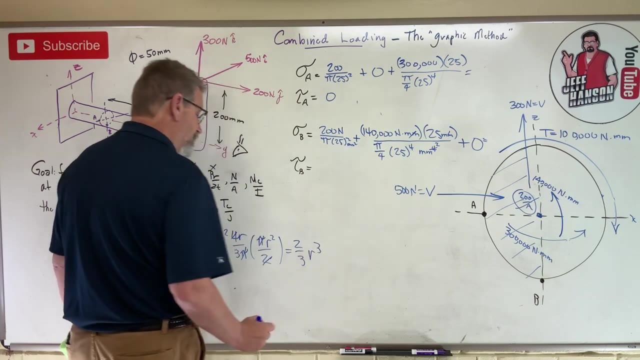 a circle Pi, R squared over two right, So what The two goes into there, two The pi's divide away And Q for half a circle always is what Two thirds R cubed right. That's a little shortcut that you can use every half a circle in the world as long as you know. 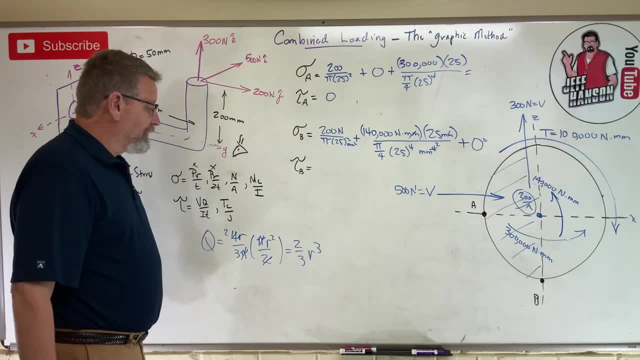 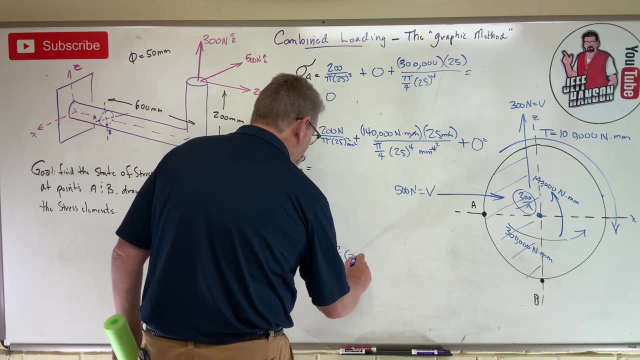 if you have a half a circle, that's the shortcut. So it's two thirds R cubed, right? So Q in this case is two thirds times 25 cubed and that's going to be millimeters cubed, okay. 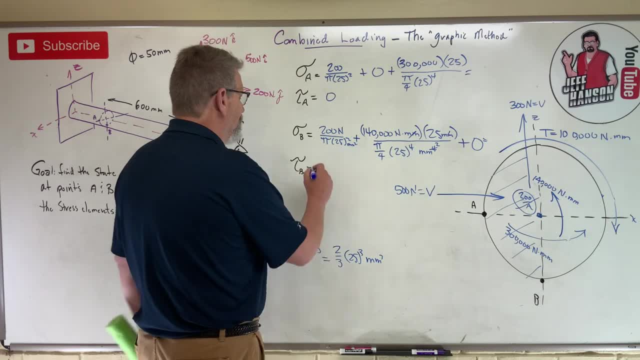 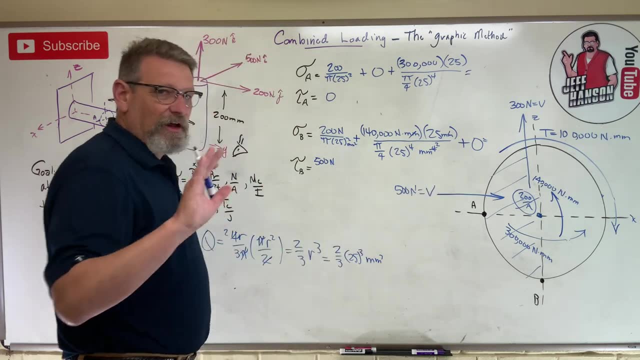 So here we go: VQ over IT. The V is 500 newtons. okay, I'm going to call it positive because it's going in the positive direction, And I'll show you a trick to sort this out. V is: 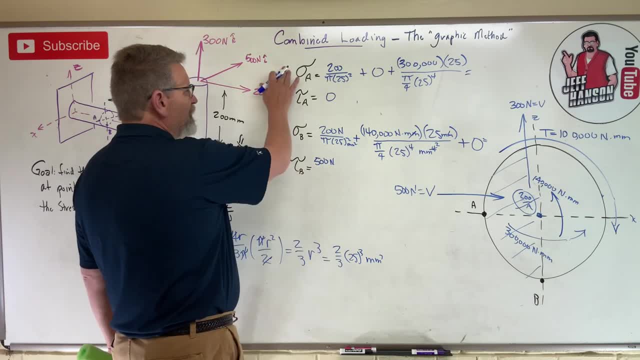 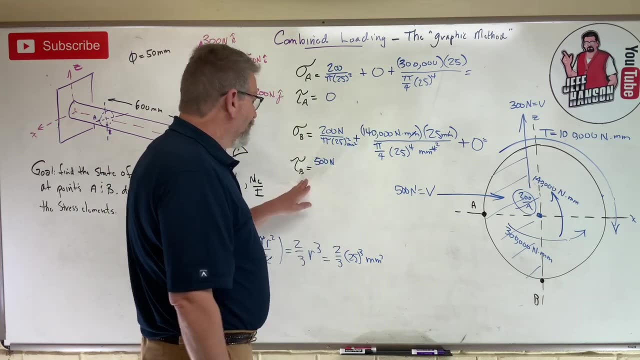 confusing on which way it goes. You know, sigmas are easy, right, If you get a positive answer, that means he's in tension. If you get a negative answer, it means he's in compression. That's easy. Tau's a little bit harder, Like: which way do I draw my tau on my stress element? Is it going up? 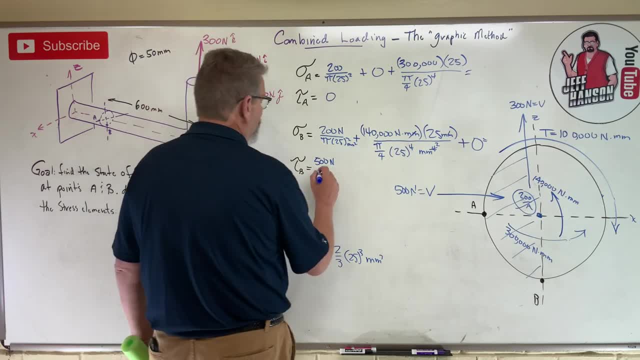 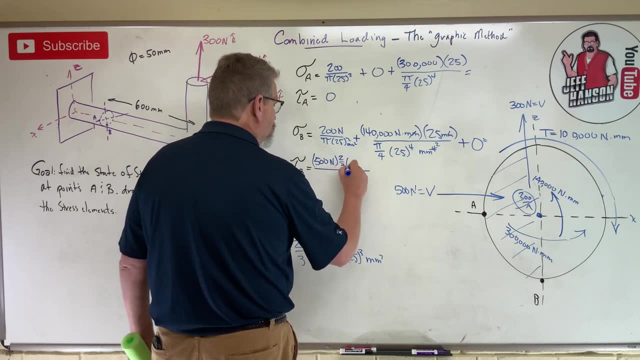 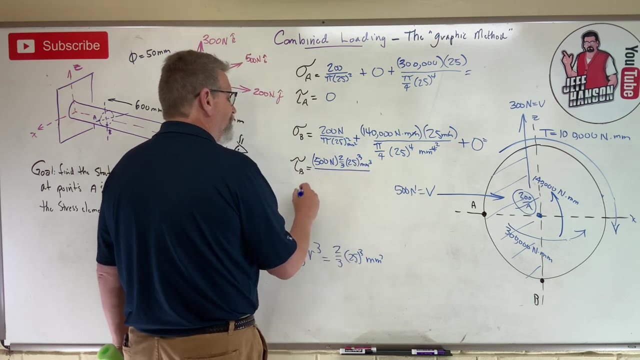 or is it going down? I'm going to show you a trick. okay, So stick with me. So VQ over IT. There's V. What's Q? Q is here. Two thirds 25 cubed, mm cubed divided by I for a round. It's the same as it was up here: Pi over 4,. 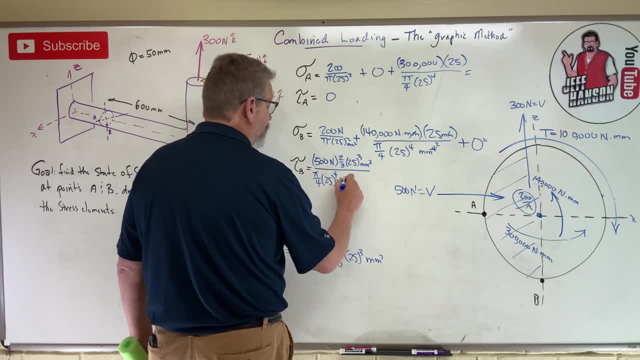 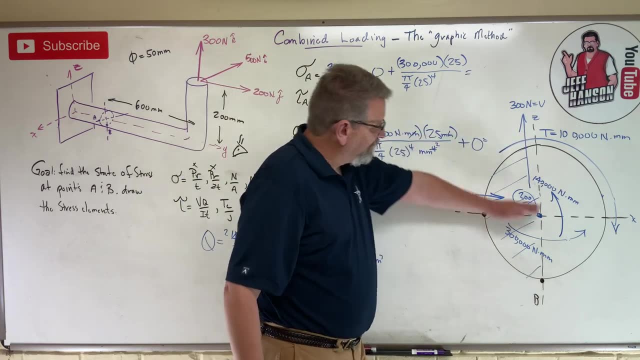 25 to the fourth mm's, to the fourth right Times T. What is the thickness? Well, it's from here to there. It's got to tear through the whole middle, doesn't it? The thickness is 50 mm's. 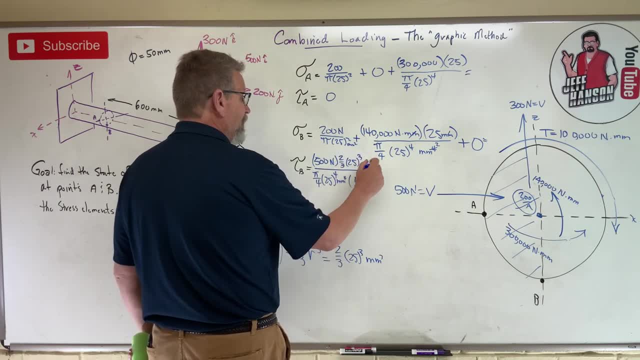 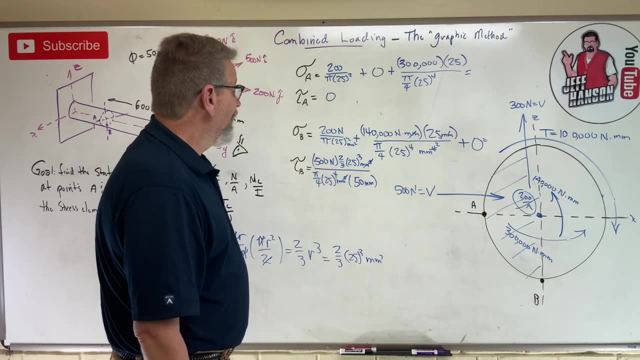 right. Look at there, There goes 3 mm. Right there, Bam, That gets 3 of those. So that leaves what Newtons over millimeter squared, That's megapascals, I know right. So I got that guy. okay, Let me move this over here. 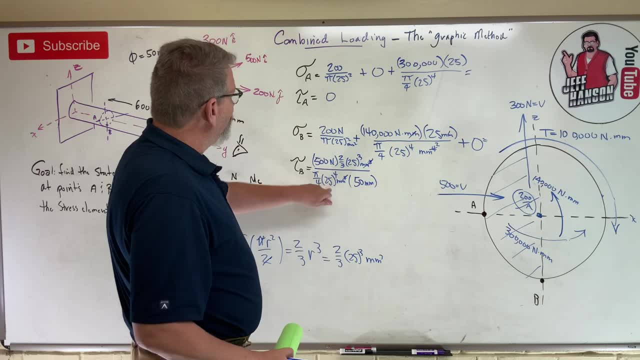 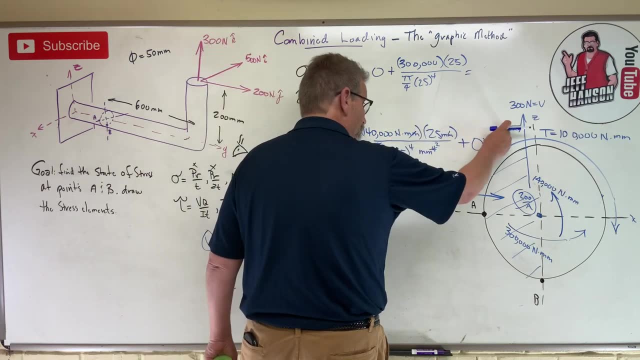 Okay, I got that guy. So that was all of that. this and that were from the 500,. right Now, we're going to do the exact same thing to the 300,. okay, We're going to do the same thing to the 300. 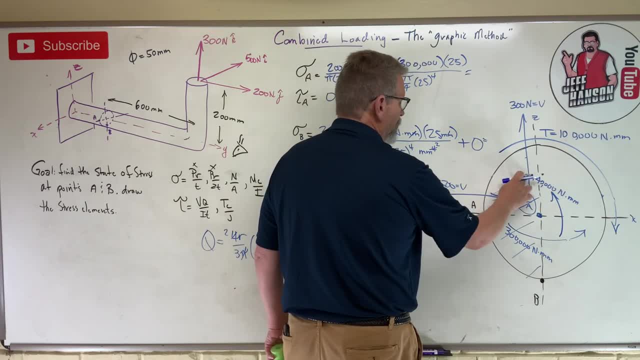 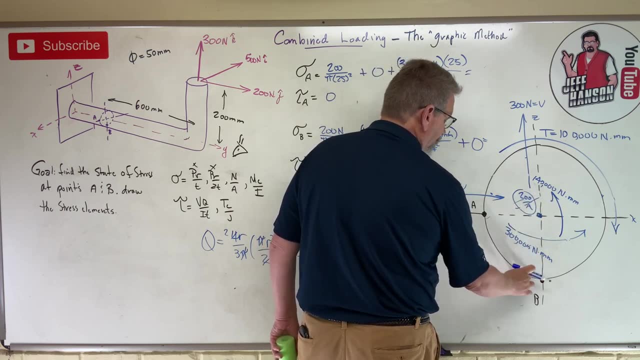 So on the 300.. Now for the 300, where's the neutral axis? Okay, Well, the force is in the Z, So the neutral axis is along the X, right, It's perpendicular. So for point B. 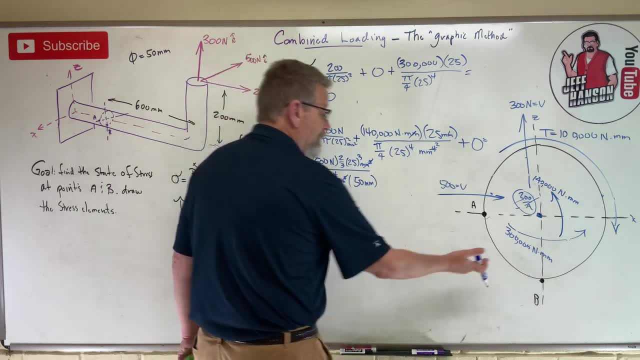 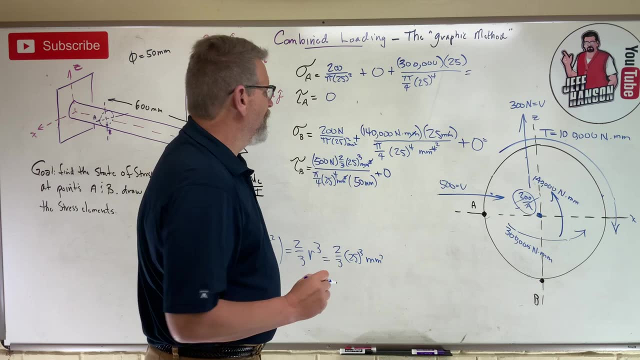 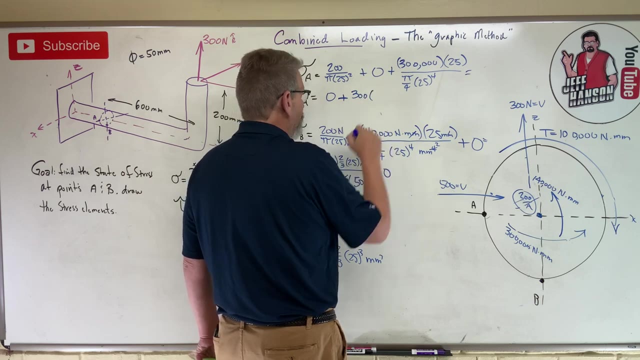 how much does the 300 make? Well, there's no area below point B, which means Q is zero, which means, boom, there's a zero right there, right. But now we have a VQ over IT for this guy. okay, So 300 times what's Q this time? Q this time is all of that. 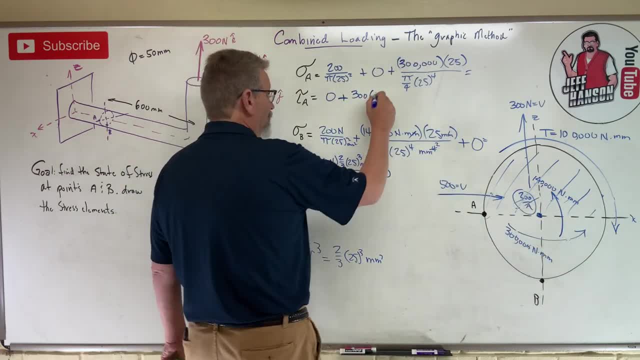 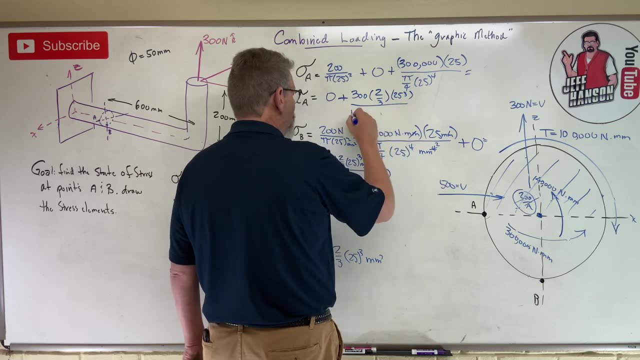 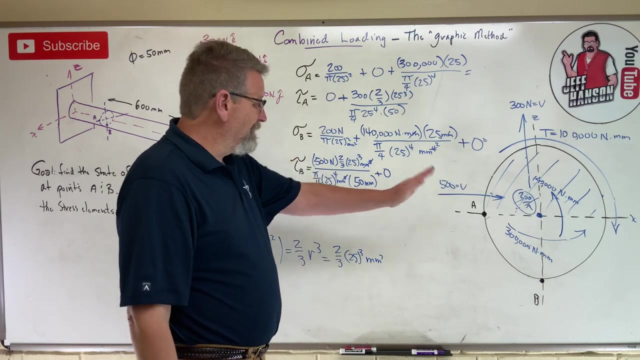 Now, that's the same as it was up here, isn't it? Two-thirds: 25 cubed divided by pi over 4, 25 to the fourth times 50, okay, Everything is the same. Everything left. Do you find this easier just going step by step and just checking everything? 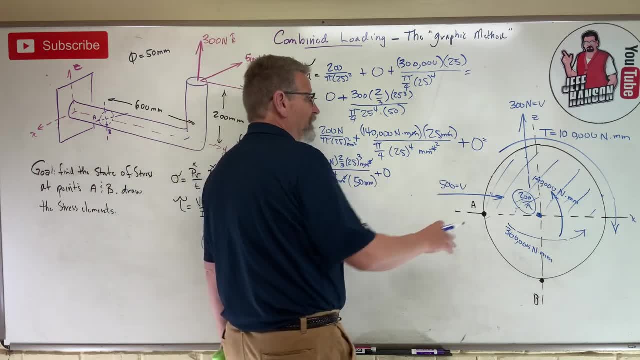 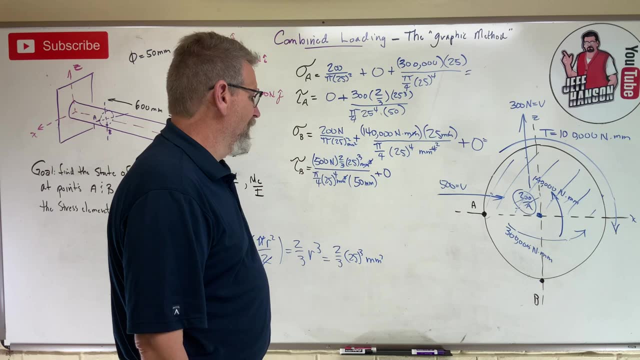 off. I mean I do. I can really see what the effects are here. The last guy is this guy right here, this T right, Which is a TC over J. Now all we got to do is follow him around, okay. 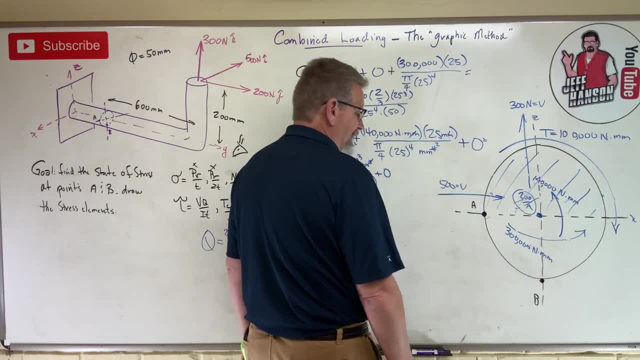 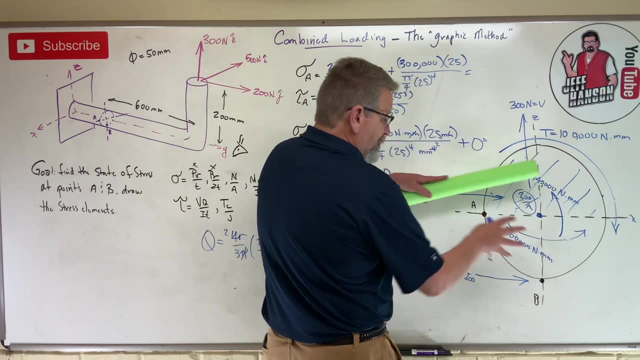 So let's go down here to point B. right quick. At point B, what do we have? Well, I had the 500 was going this way, didn't I? There's the 500, right, All the shear force is in that direction. 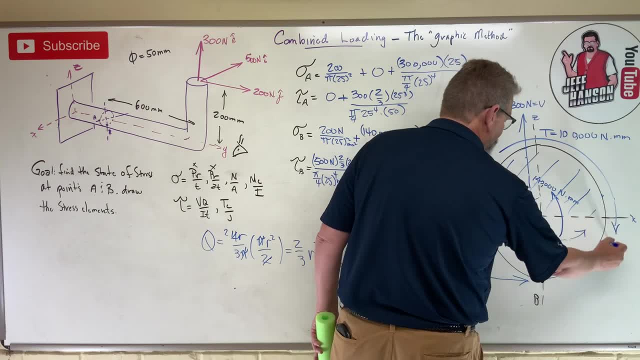 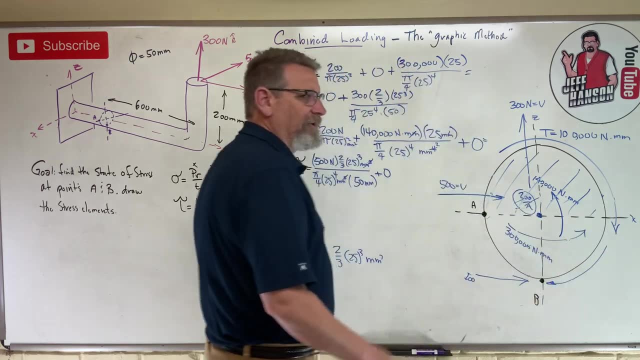 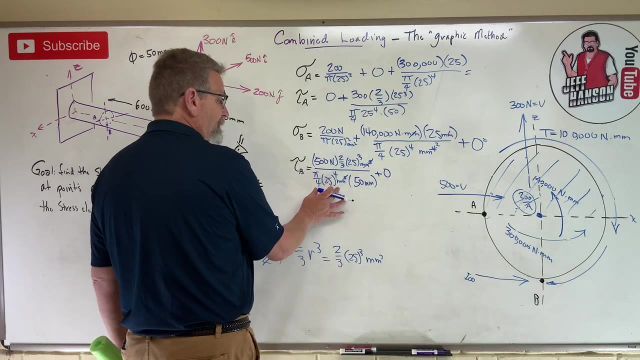 right, Let's follow T around. What's he going to do to the 500? Bam, The 500 went that way, but the T is going that way. What does that mean? That this is going to create opposite shear from that right. So if we call this at point B, if we call that positive this, 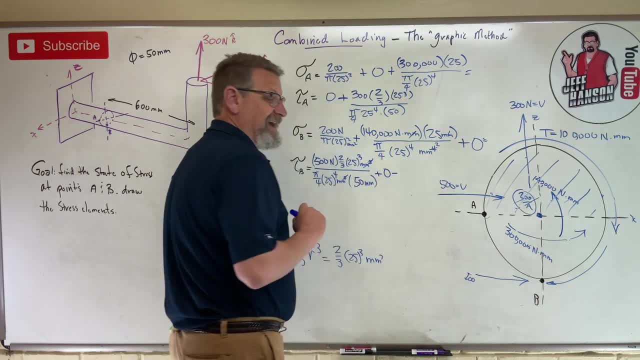 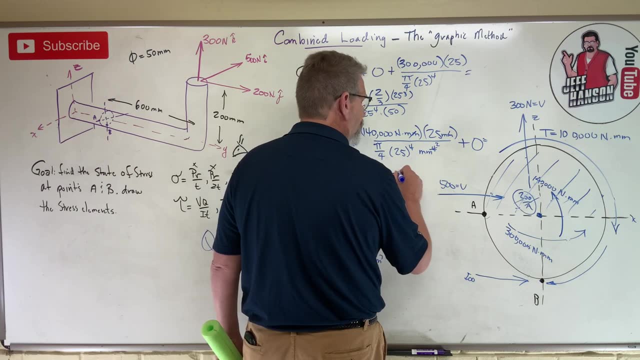 next little bit: the TC over J needs to be negative. You with me on that? Okay, so let's do that right quick. T: how big is the torque? 10,000 newton millimeters, right, No, 100,000. 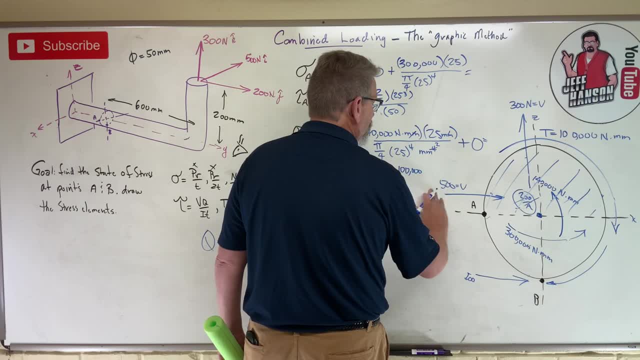 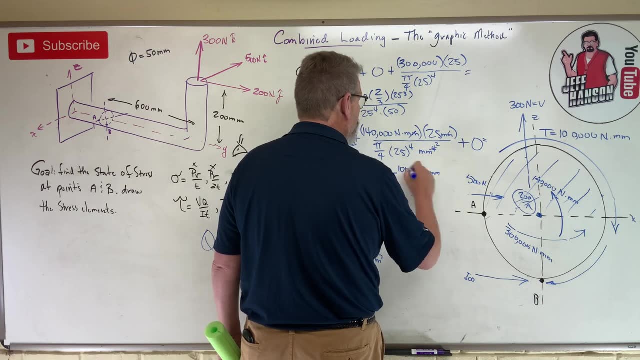 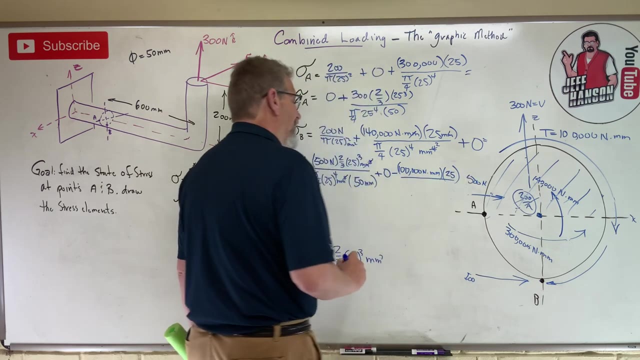 Okay, 100,000, 500,. you're still in the way. Okay, 100,000 newton millimeters TC over J. What's C 25,? okay, over J. The polar moment of inertia, not to be confused with I which. 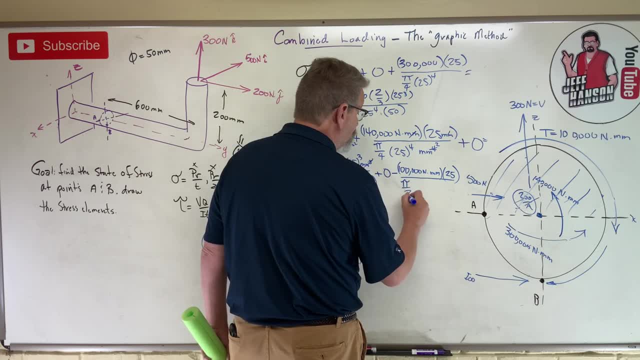 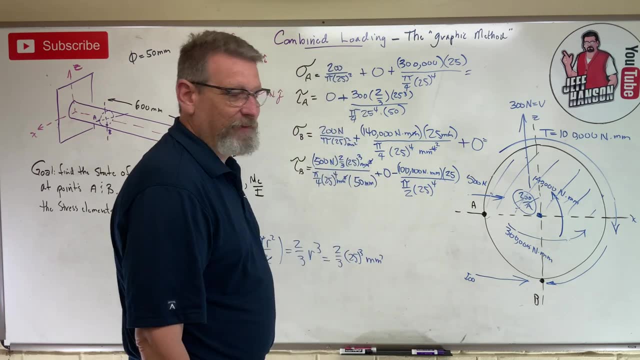 was pi over four, but J is pi over two. R to the fourth right. Okay, it's very similar. That's an easy thing to mess up, isn't it? Okay, so this one's positive, that one's in the opposite direction, because the torque falling around boom is. 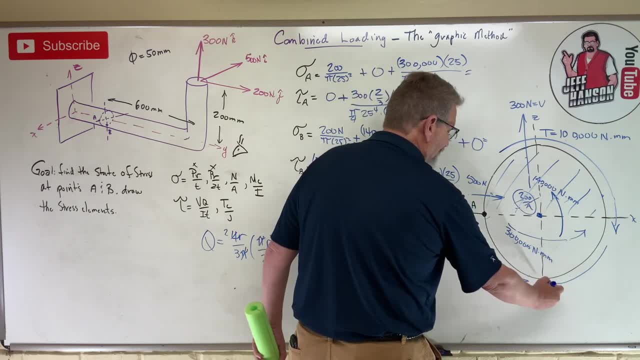 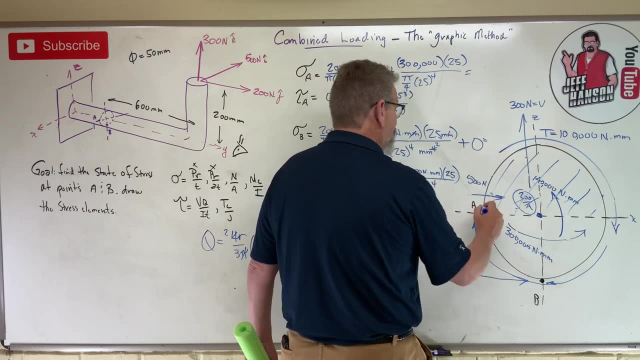 pushing on B that way, right Now, let's follow him on up to A. Okay, here he comes. Okay, pushing up on A, isn't he? Well, what was 300 doing? The 300 was going upwards across. 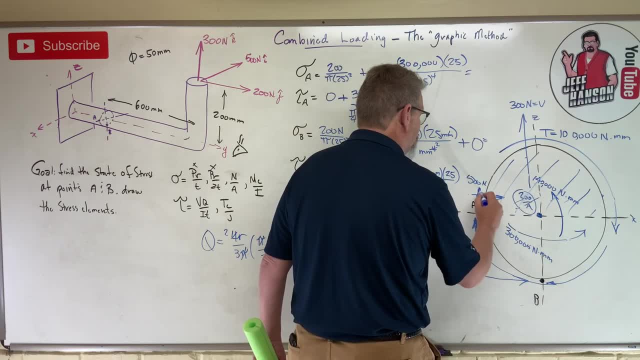 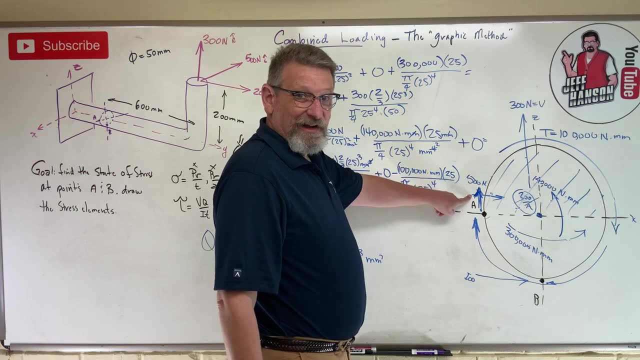 there, right, The shear was upwards. So the shear was in this direction from the 300.. So what does that mean? That the TC over J shear is going to be positive. The T shear is going to be in the same direction as the BQ over IT shear was right, They add. 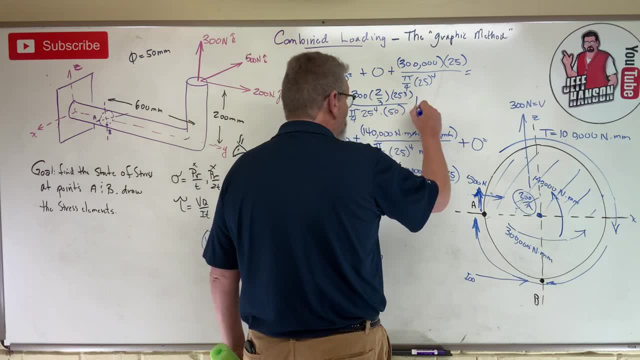 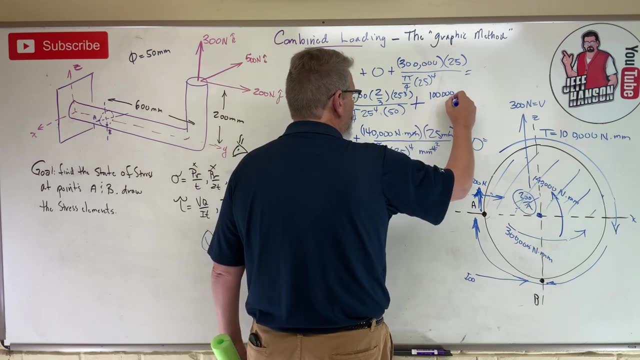 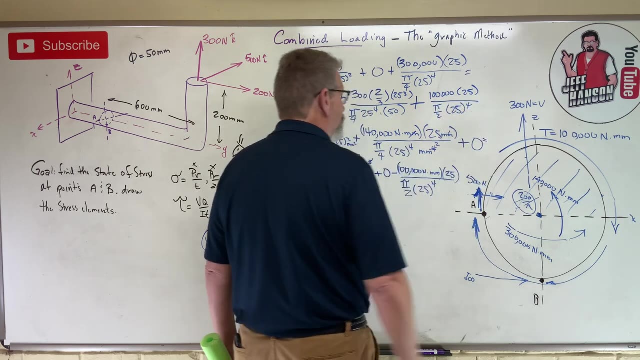 together. So let's go up here, right, This one's going to be plus same amount, right? Same thing: 100,000 times 25, divided by pi over two. 25 to the fourth, okay, And that's. 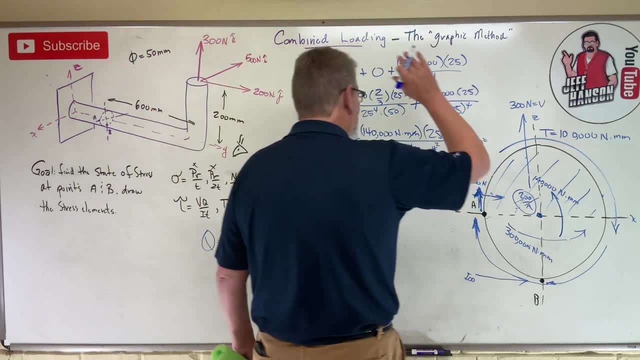 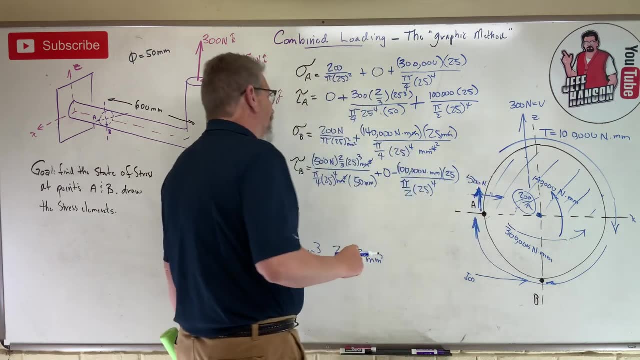 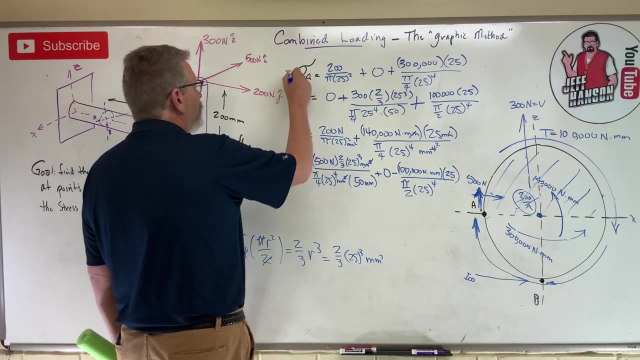 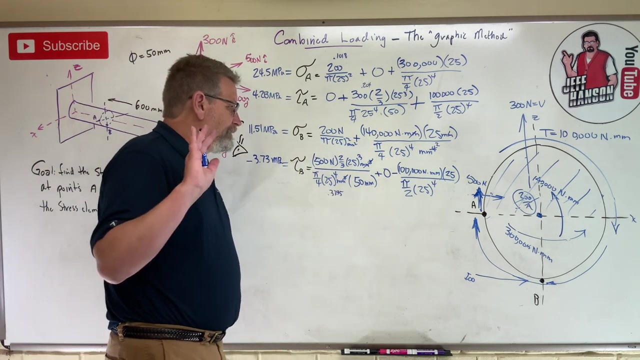 it. So the next thing I got to do: I got all my equations written. I'm going to do this, I'm going to go ahead and put this in my calculator and then I'll tell you what I get for sigma A, tau A, sigma B and tau B. okay, Here I go. Okay, we're back All. 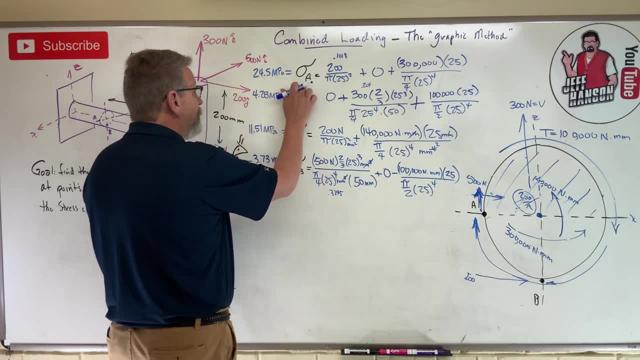 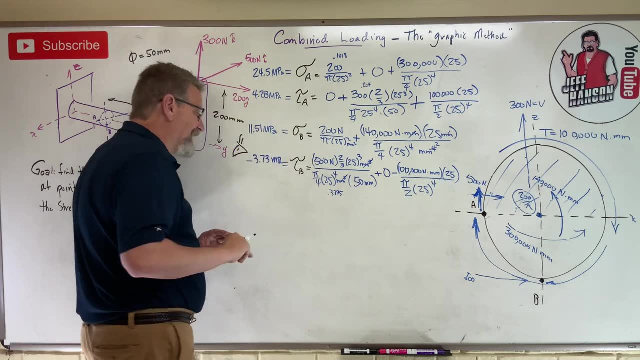 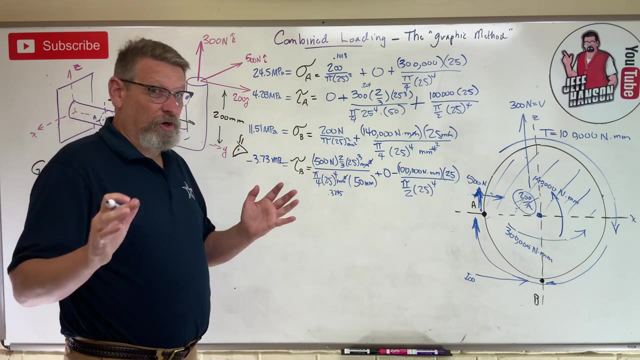 right, I got these answers. I got a positive: 24.5 megapascals for A. positive: 4.28 megapascals for tau A, 11.51 positive for sigma B. Negative: 3.73, negative: 3.73 megapascals for tau B. So what do we do here Now? how many? 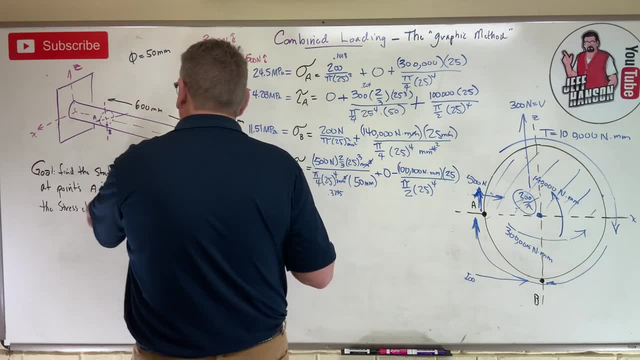 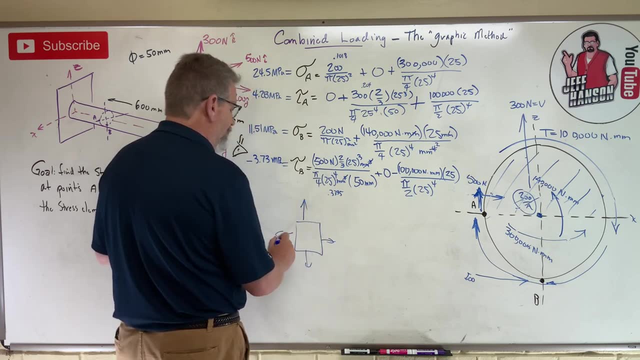 of you think, or had a thought, that I could draw one stress element. right, If I drew one stress element and then, like, A would be in this direction and like, maybe B would be in that direction, right, Right, I can use this sigma for one of the sides and I'll. 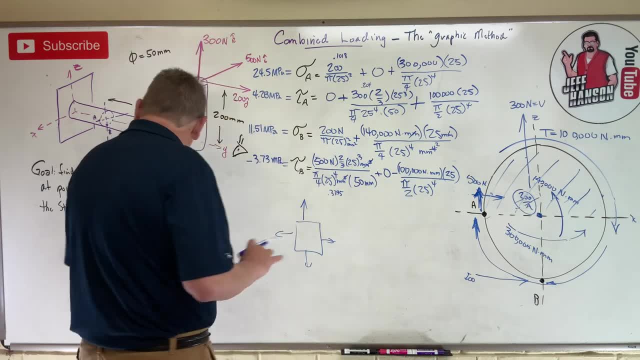 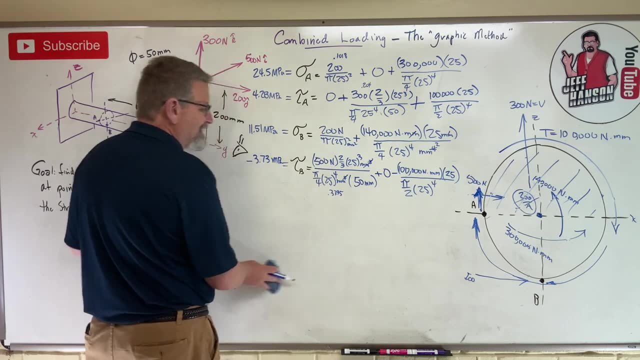 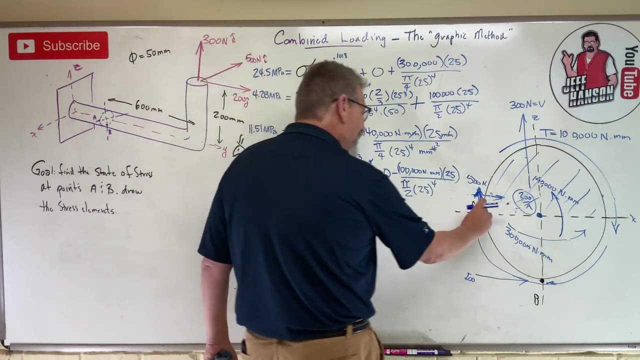 use that sigma for the other. No, no, no, no, no. Why is that not right? Because A would be here at completely different points. Remember, a stress element is an infinitesimally small little area, a little patch there on the side right, And what's going on at A is totally. 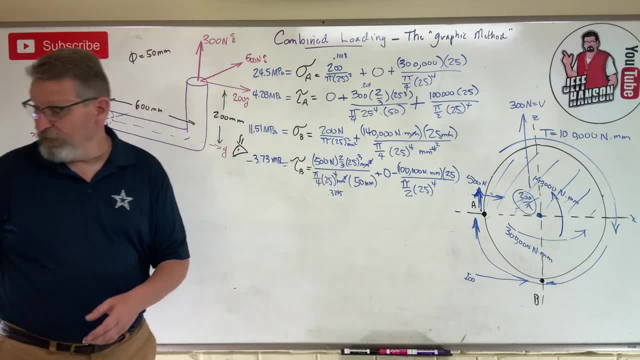 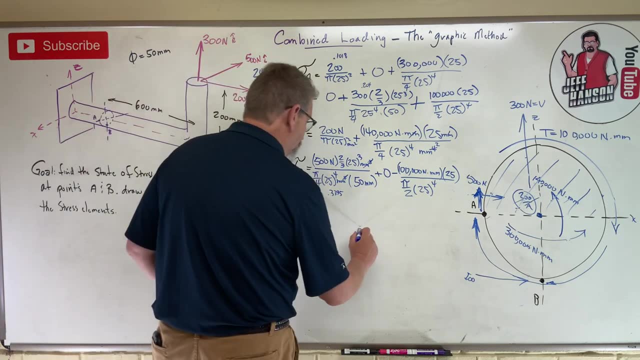 different than what's going on at B, So I got to draw two separate stress elements. okay, So let's do this. Here's one for A. okay, Here's A. and here is B- okay, B. So. 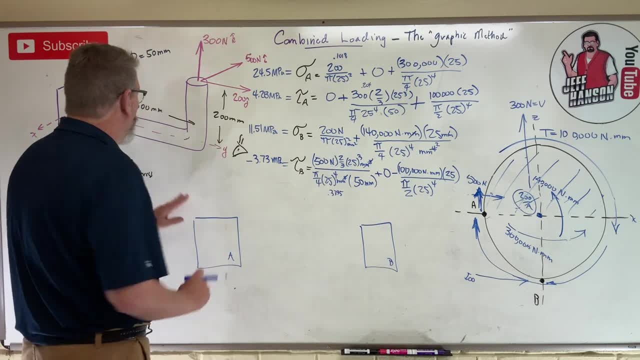 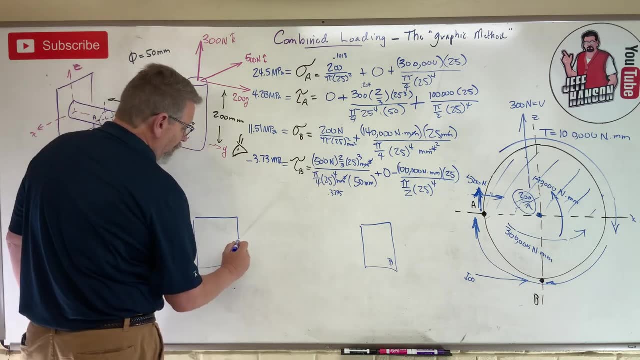 the sigma stress number one, right, All of the stretching from bending and from pulling or whatever is along the Y axis, right? So it would be like along this way here, right? If I'm a little piece of, I would feel. 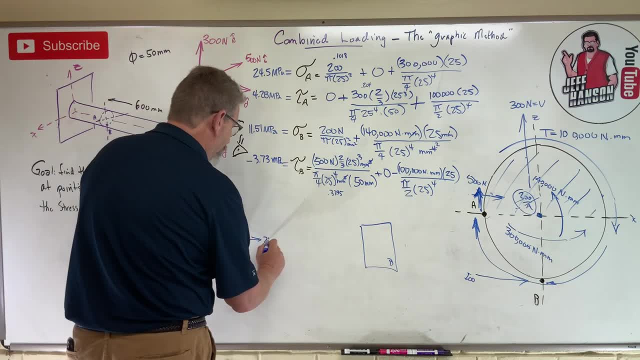 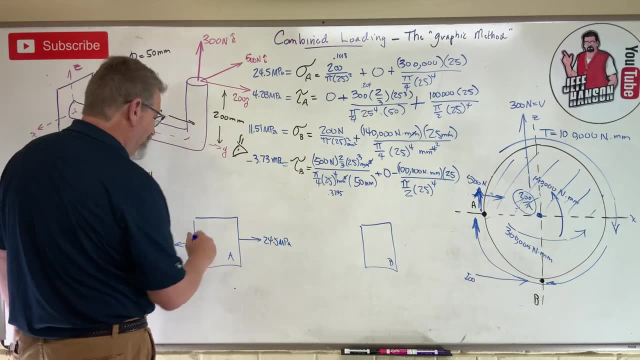 this right Positive. So for A, I feel 24.5 megapascals, right. What do I feel in this direction? Nothing, zero, right. Same for this guy. I would feel this If I'm at B. 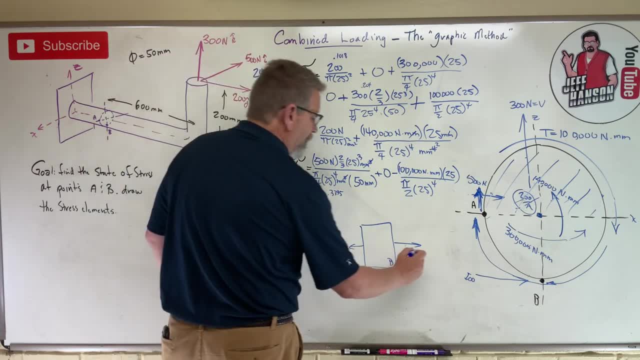 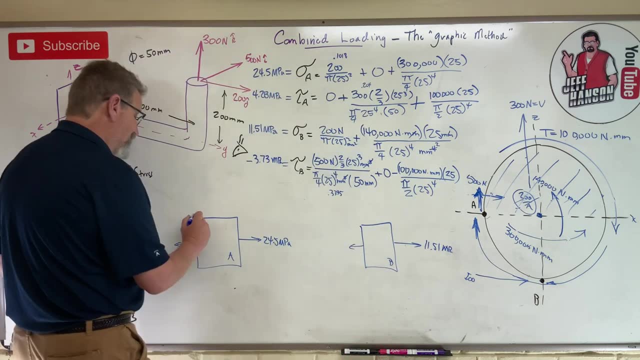 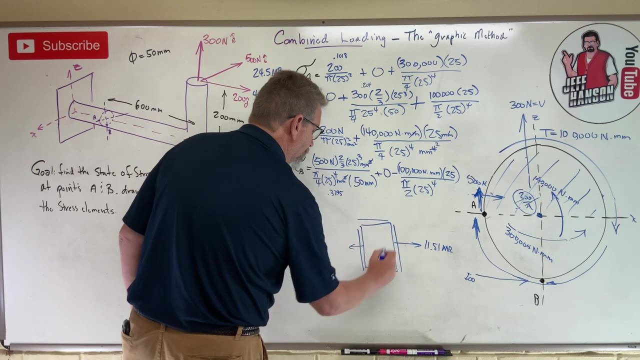 I'm on the bottom, I'm still positive, but I feel 11.51.. Okay, So the question then becomes: here's my taus, right, Here's my taus. Now I know for a fact- right, I can look at these taus- that they're going to be going opposite on. 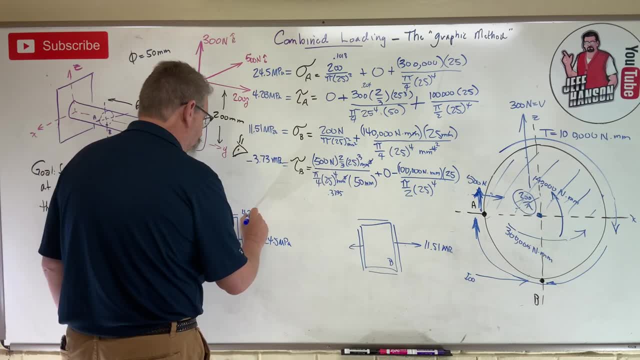 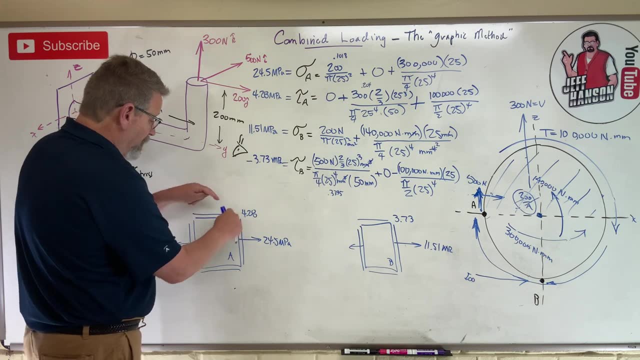 B than they do on A right. So this is 4.28, and this is 3.73.. But the question is: do they go to this corner or do they go down? I don't know. This is super confusing. All I've got to do is figure it out from one point. 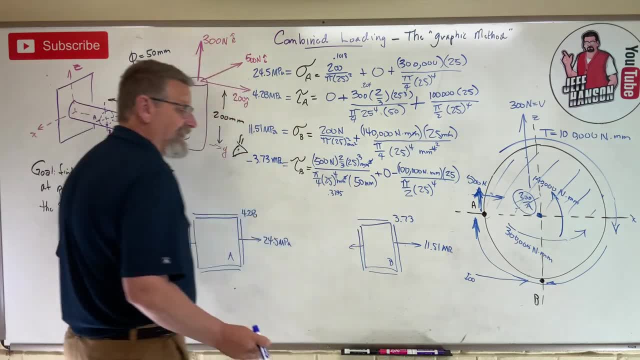 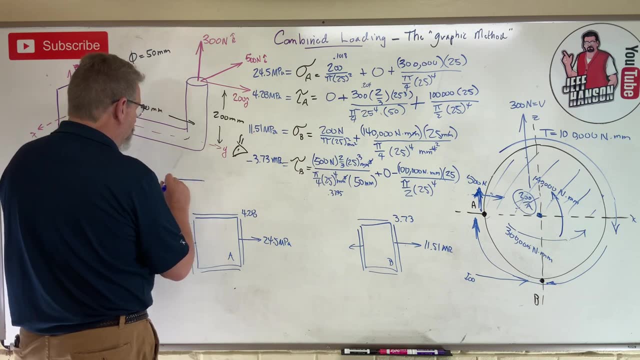 If I know one, I know the other one, Because the sign was negative, it's going to be the other way, So let's do this. Look here, If I'm at point A, let me draw this from the side view. okay, Here's side view. I'm going to draw it like this: okay, Whoop. Okay, there's. 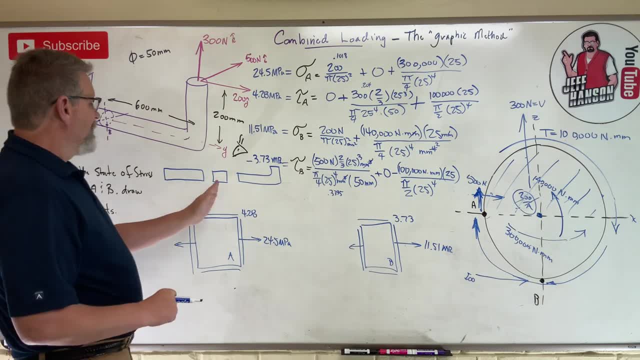 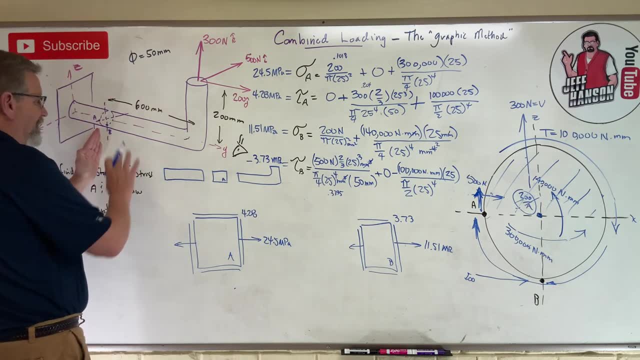 side view of my pipe-looking deal. What I've done is I chopped it in half and there is point A right there, right. So I sliced my beam whoop in half, right there, and I got this part. I got my little. 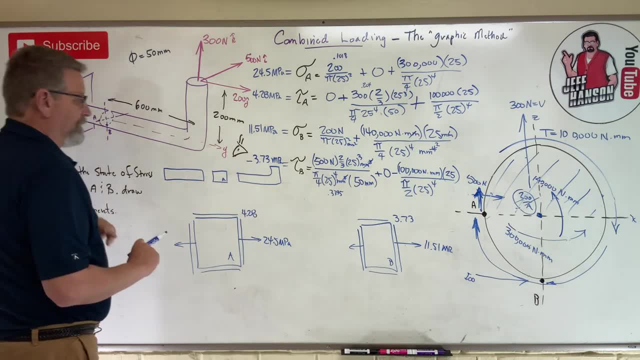 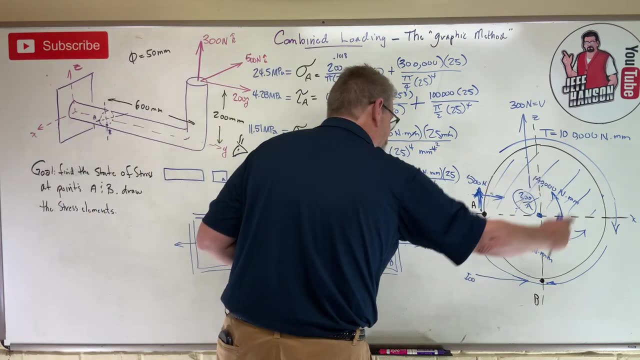 stress element. there he is, and then I got the back part of the beam right. So let's look at point A. What did I get right? I drew these as positives. So they're going upwards right, So the net is upwards right And I got a positive answer for that tau. 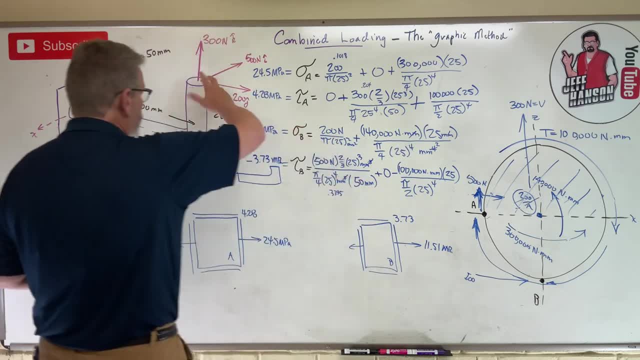 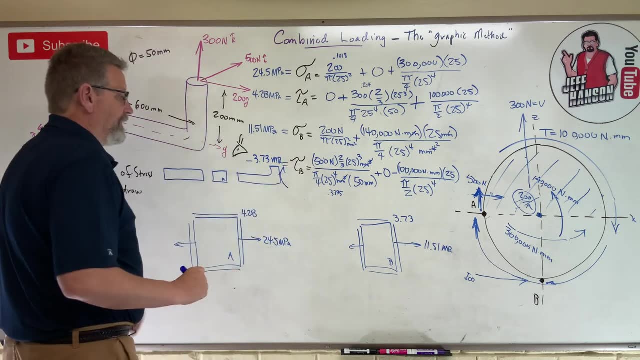 So I know that the net of the torque on the whole thing is going to be a torque like this, There's a torque like that, There's a force like that, right, If you look at this here, right From the torque, from. 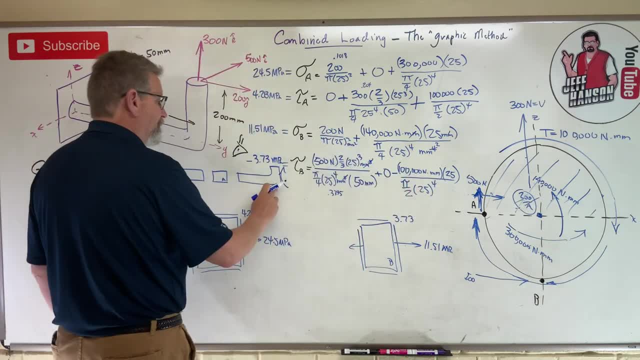 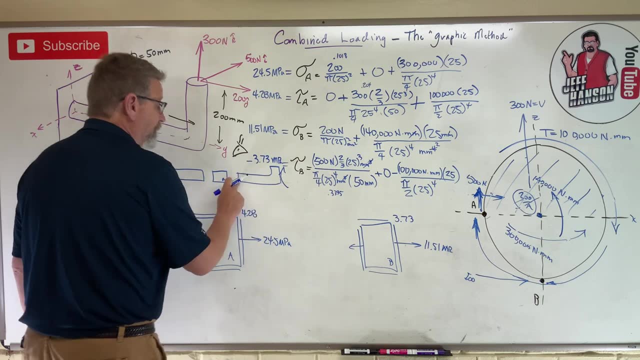 this force and from the sheer force. right, You get that That's all going upwards, right? So there he is going upwards. That's from the force on the end of the beam. So over here I cut it. What has to happen? Well, it's got to go down. So what? on my stress element. 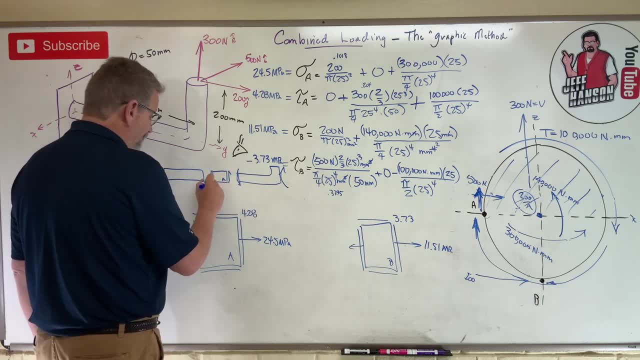 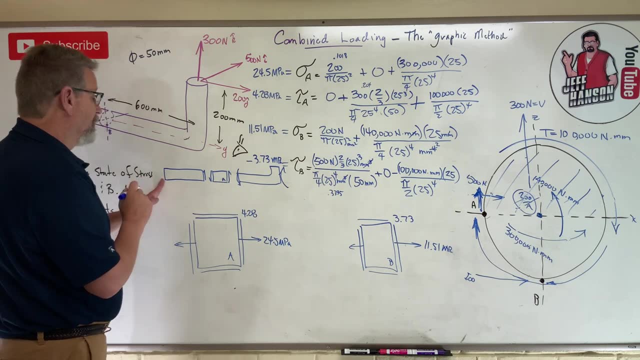 Got to go up. So what on this side of stress element Got to go down? So what on that side Got to go up? and then what about over here at the end of the world at the reaction at the wall Right? 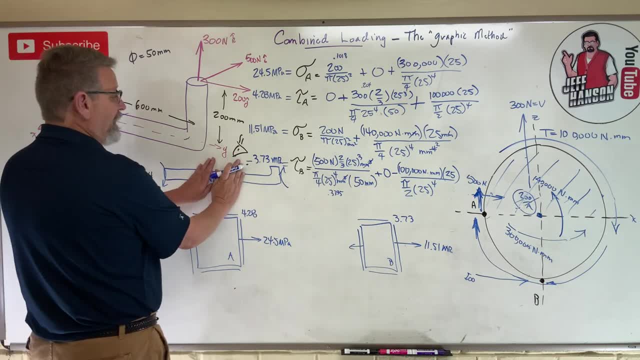 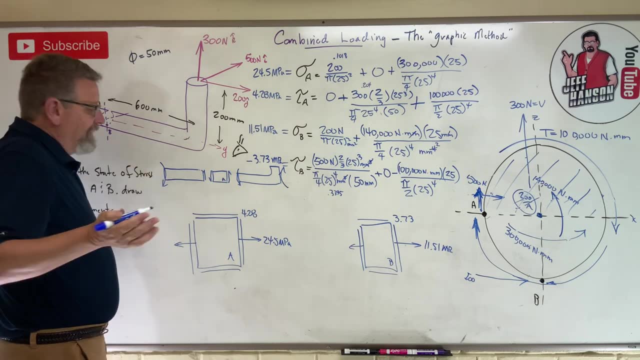 right Got to go down. So look at the whole thing. Take this away. If the net was a positive rotation- you know this way- then this has to be a reaction, the opposite direction. That makes sense to me, doesn't it? So do you see what I did? I just sounded out to myself what that stress. 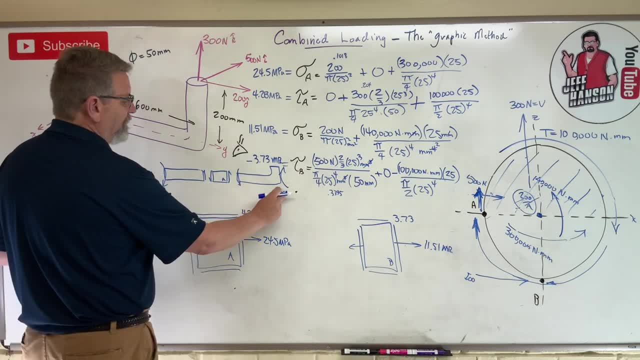 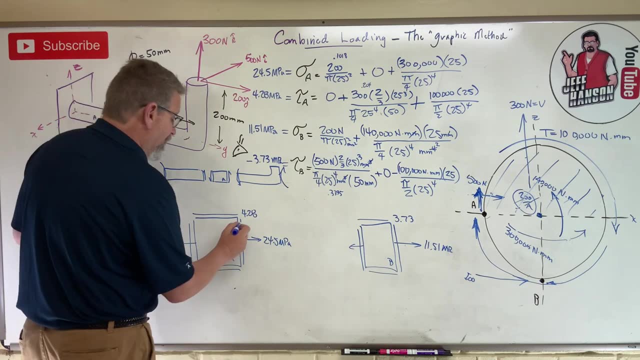 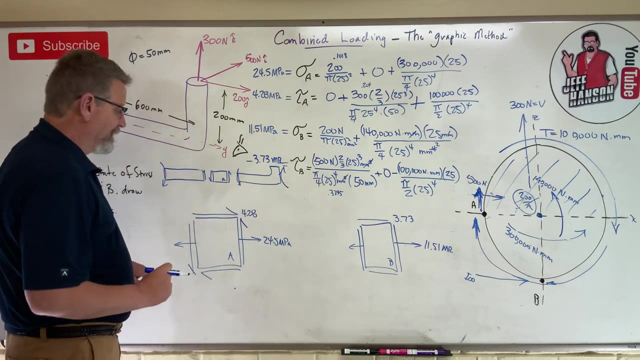 element. Now here's another little secret: If this is up, this side is always up. If this is down, this side is always down. There's your little shortcut, right. So here we go: This is up, This is down, And we know those come together at the corners: Boom right. And so there's my 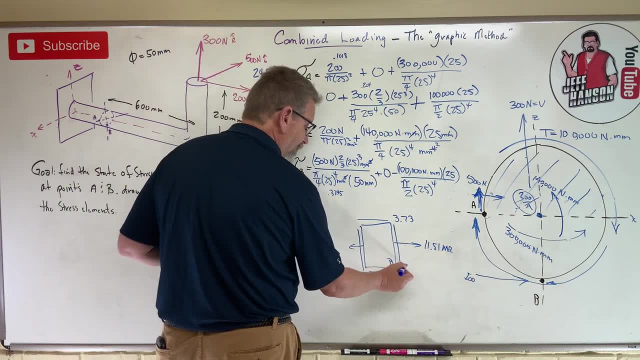 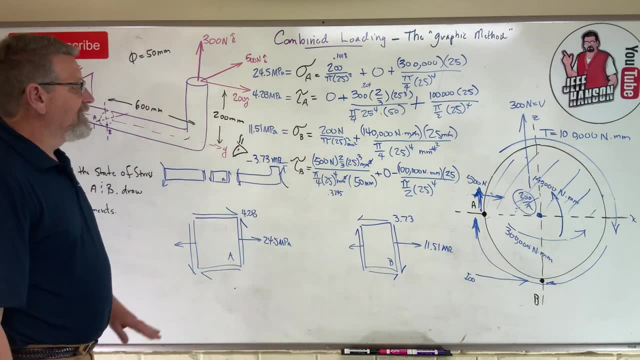 tau. And then over here, what do I have Got to be opposite of that, doesn't it? Uh uh? and then uh uh, There you go. Stress element A. stress element B. The graphic method: Sketch the cross. 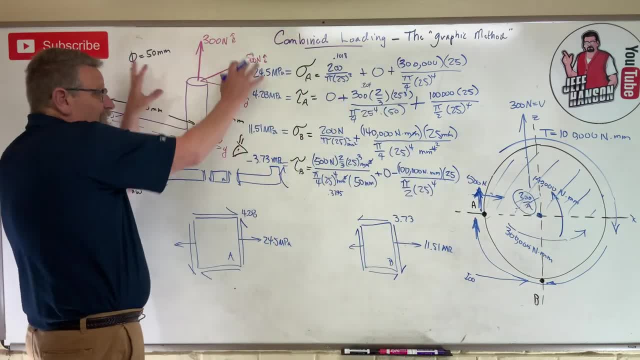 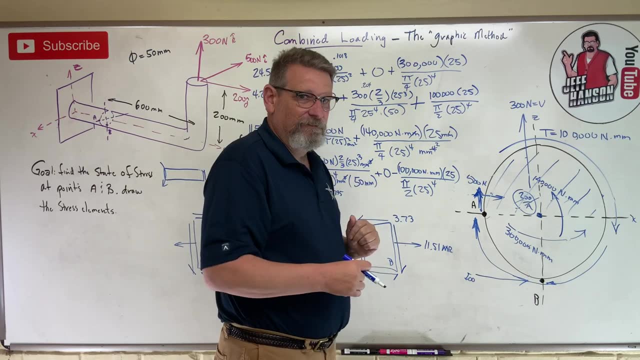 section right. Sketch all the effects from the forces on the thing, whatever it is. Is it torques? Is it moments? Is it whatever? right? Sketch all the effects On the cross section And then carefully go through it, one at a time, and write your equations.